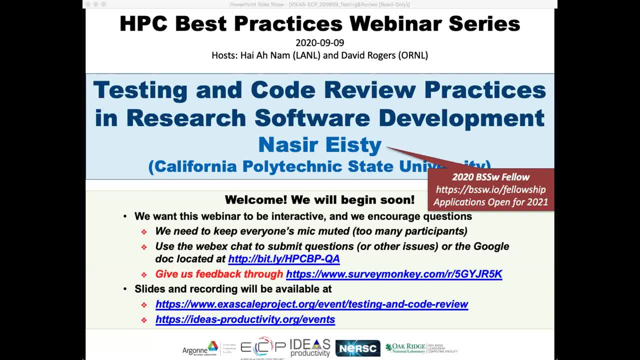 in Research: Software Development. The webinar is going to be presented by Nasser Eisti from California Polytechnic State University, So Dr Eisti is an assistant professor in the Computer Science and Software Engineering Department of Cal Poly, San Luis Obispo, And 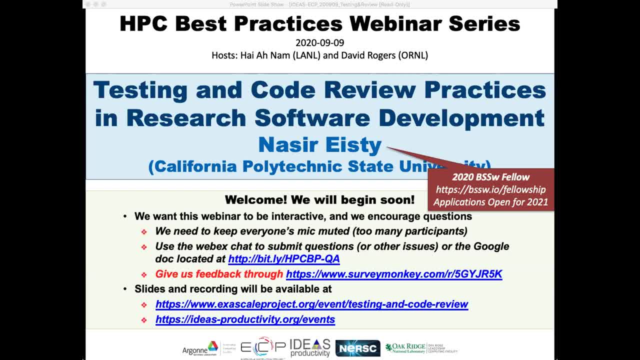 he received his PhD in computer science from the University of Alabama in spring 2020.. His research interests lie in the area of empirical software engineering, software quality and research software engineering. Dr Eisti has prior experience working at Los Alamos National Lab and the National Center for Supercomputing Applications, NCSA. He 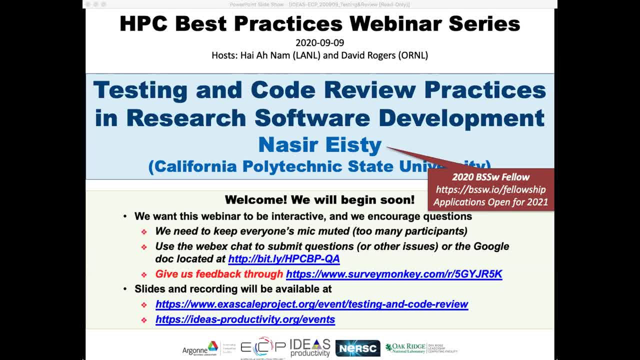 is a recipient of the BSSW 2020 fellowship. Dr Eisti is a graduate of the College of Energy Fellowship Award from the Department of Energy, So I'm going to stop sharing my screen so that he can start sharing his While we're. 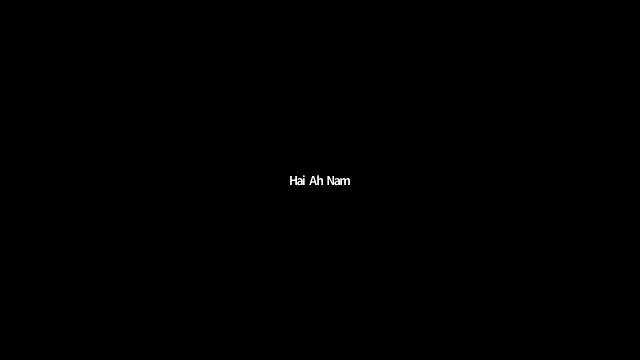 doing that. I just want to remind everyone that we have over 200 tickets for this webinar, so all attendees have been muted upon entry. If you have a question, please enter it into Zoom chat. So the Google Doc linked in the Zoom chat, so I'll link it one more time for the new. 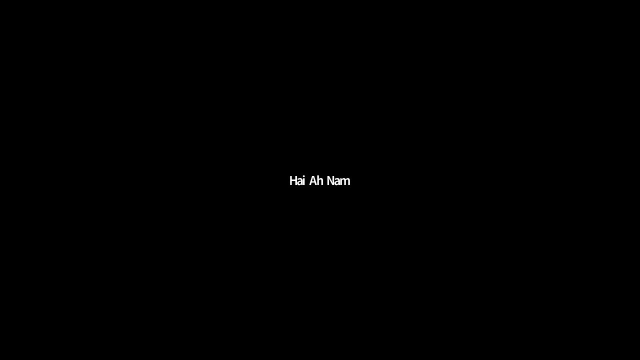 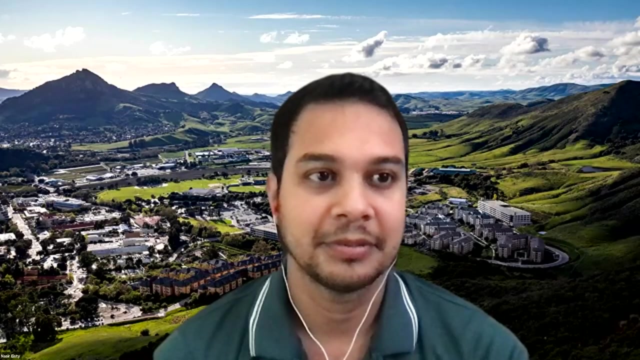 folks And Dr Eisti will take breaks periodically so that we can respond to any questions that come in. So with that now, Sergio, do you want to go ahead and share your screen? Yeah, Oh there, you are Wonderful. So we're going to go ahead and share your screen. So we're. 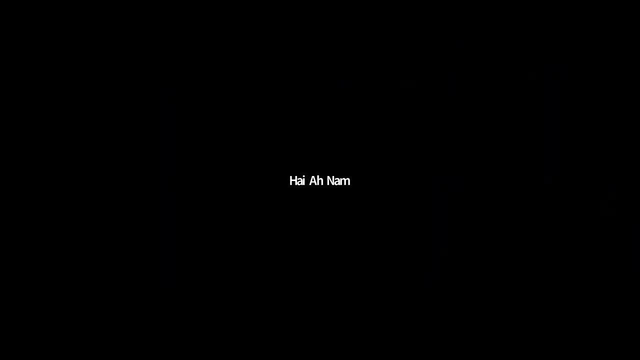 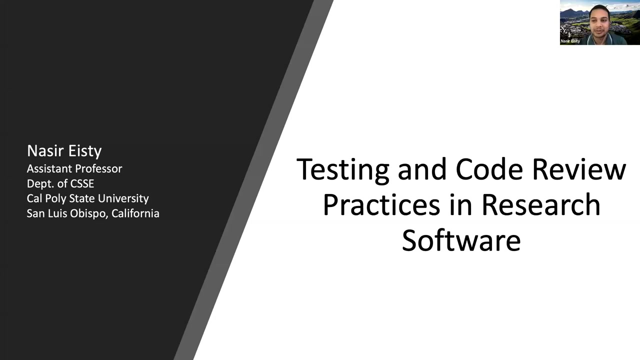 going to go ahead and share your screen, So with that, I'm going to go ahead and hand it over to you. Sure, Thank you. So welcome everyone to this webinar on the current practices of a couple of software quality activities- testing and code review in research software development. 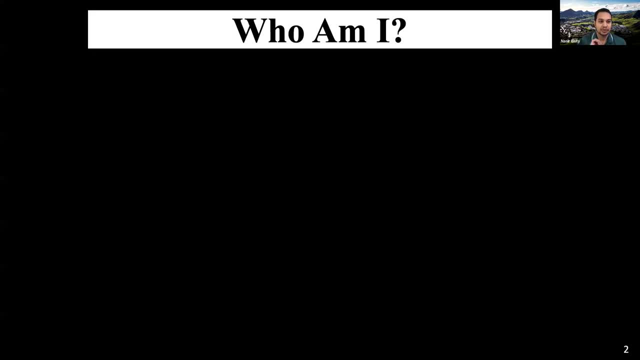 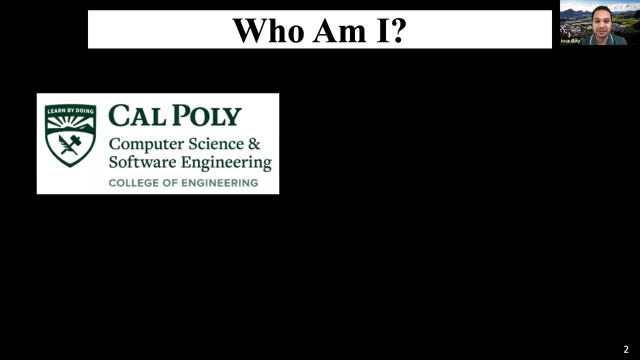 Yeah And Okay. So here already he introduced me, and thanks for doing so. Yeah, I'm a brand new assistant professor joining this fall at the California Polytechnic State University in the computer science and software engineering department, And I graduated my PhD from computer. 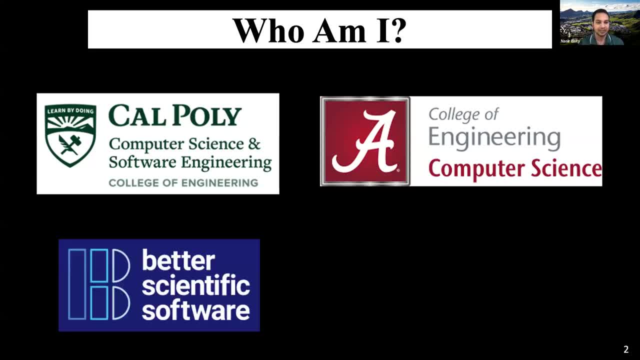 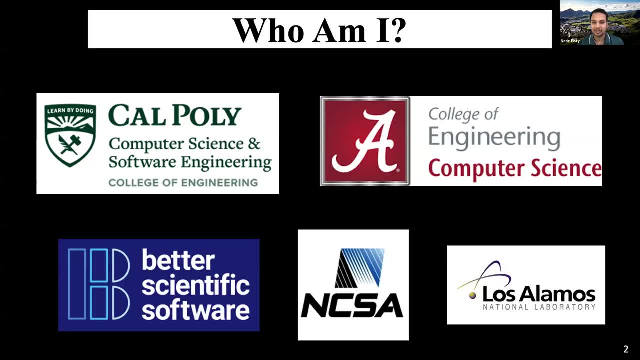 science department in the University of Alabama And, yeah, I'm one of the BSSW 2020 fellow and I have prior experience working at NCSC and Los Alamos. Okay, So my research focuses on empirical software engineering and software quality. assurance. 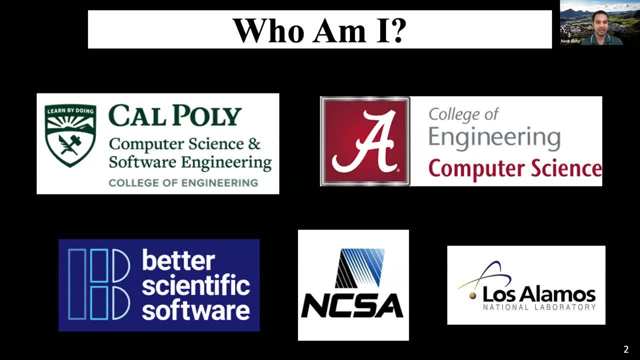 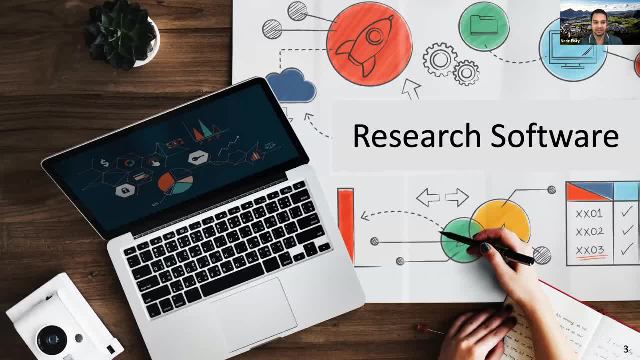 especially in research software. So what is research software? Research software is a special kind of software developed by researchers from a wide variety of domain, including, but not limited to, science, engineering, business and humanities. Researchers develop software to make predictions. This is a kind of software that solves computationally complex or data-intensive problems. It can 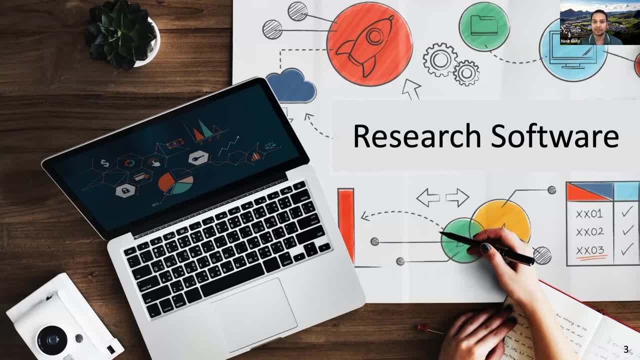 range from large physical phenomena around on high-performance computing machines, such as simulation software for nuclear industry, medicine and the military, and to smaller simulations and developed and used by groups of researchers on a desktop machine or a small cluster. Sometimes this category of software can be used to solve complex or data-intensive problems. 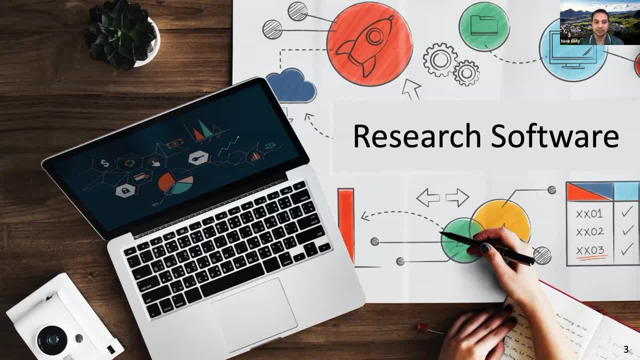 For example, if you have a computer that has a computer that has a computer that has a computer that is on a desktop machine, it can be used to solve complex or data-intensive problems. The next category of software provides infrastructure support, That is, messaging, middleware, scheduling. 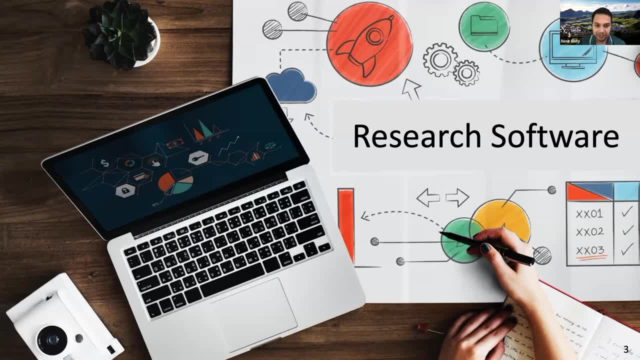 software or libraries for mathematical and scientific programming. Research software is also used in computing evidence for research publications and we call research software developer to any researchers who develop software. They can range from researchers who do not pose any software engineering knowledge to experienced professional software developers. 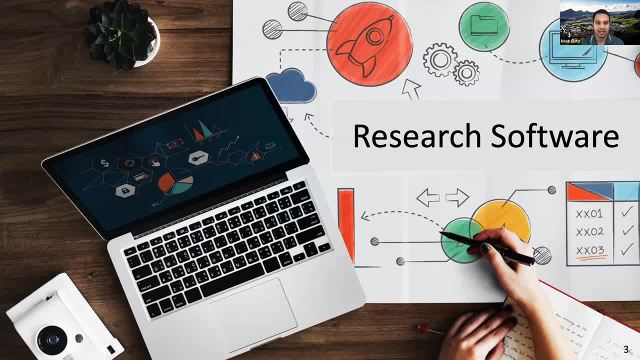 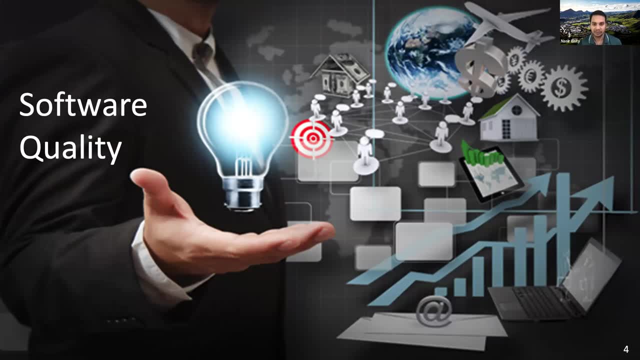 with considerable experience, software engineering knowledge And researchers draw insights and make critical decisions based upon the results obtained from research software. So therefore, the correctness of the design and implementation of this software is of utmost importance. If the software is of low quality, the results are less trustworthy and 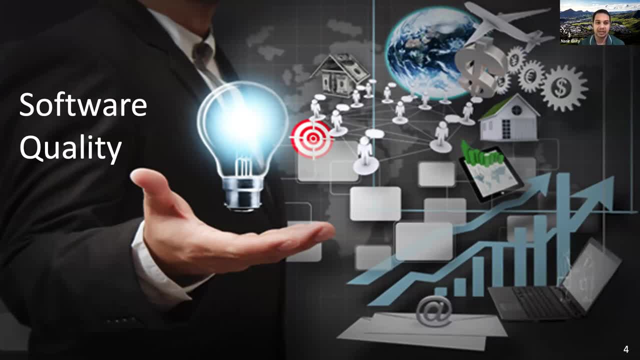 then prone to failure in mission critical situations. So low quality software may lead to incorrect research conclusions as well. But it is very difficult to make the research software error free because of the complexity of the underlying science, relatively unknown results from scientific algorithms and the constantly growing esteem of data. 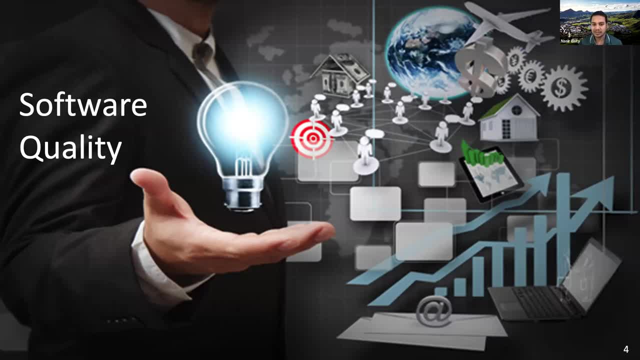 And we have also observed that researchers often place less importance on traditional views of software quality than on other scientific goals. So, regarding this impact, my research focuses on developing techniques and tools to assist developers in efficiently building high quality software. So today I'm going to present the results from 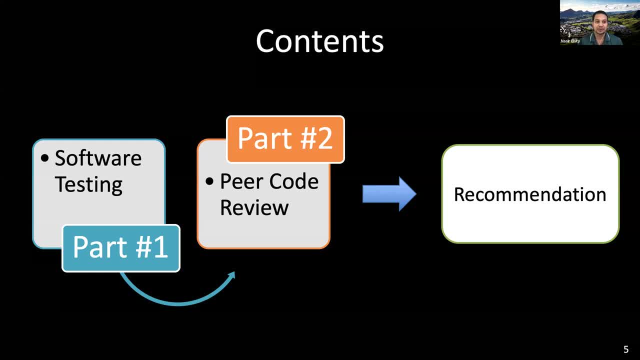 two community surveys, So I'm going to show you tons of charts, So be ready for that. And in the first part of this survey I will talk about software testing And in the second part I will discuss code review practices in research, software development And. 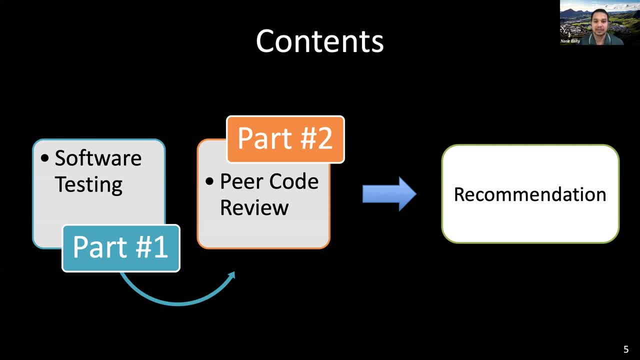 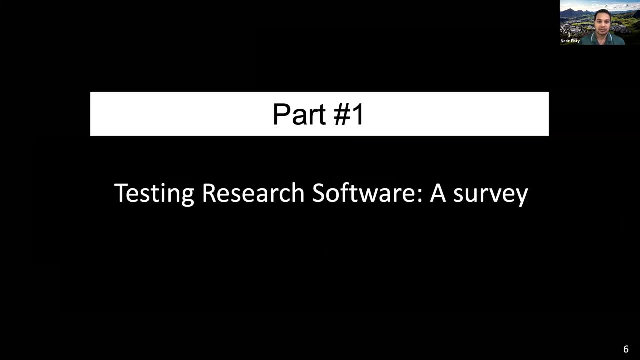 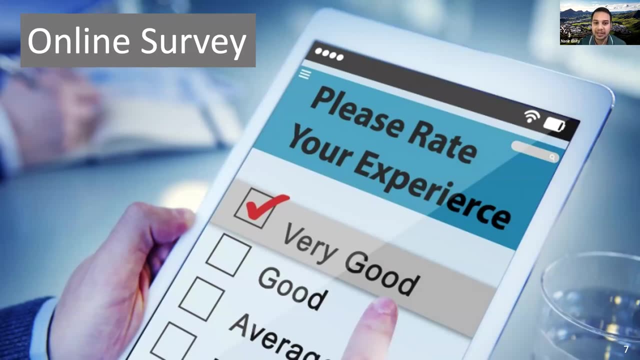 then at the end I will provide recommendations for best practices of software testing and code review in research software. So jumping into the first part. So we conducted an online survey. So at first we piloted the survey directly with some experienced research software developers and adjusted the wording according to. 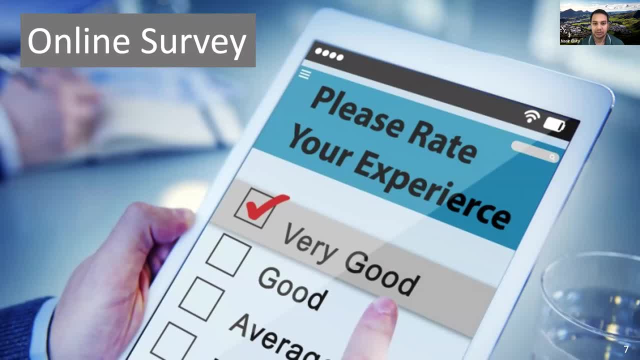 their suggestions to make it clearly understandable to the respondents, And then we made sure that we provided enough definitions so that the software engineering terms used in the survey do not create any confusion to the respondents. We also have the IRB application approved from the University of Alabama, And then we sent the survey out. 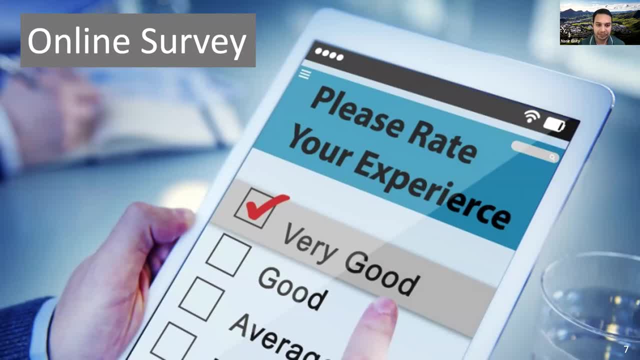 to mailing lists of research software developers. We circulated the survey to RAC research software engineering Slack channels across different countries around the world And then some of our collaborators spread the survey through different Department of Energy national laboratories in the USA And in addition we published the survey in the monthly newsletter of. 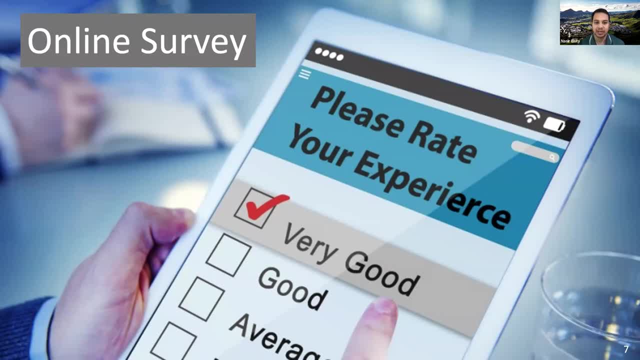 Better Scientific Software, BSSW and IDeA's productivity mailing list, And we have used a tool called Qualtrics to develop the online survey And we kept the survey open for about a month And at the end of the survey, 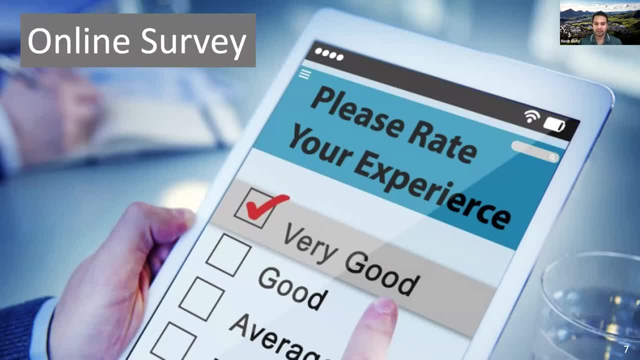 I was able to gather 120 complete responses to include in this study And for the data analysis I used the tool SPSS Programming Language R to analyze the quantitative data And for any data that are qualitative. so both me and my PhD advisor individually quoted the data. 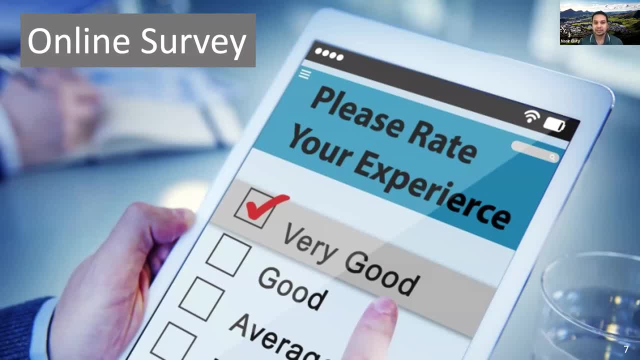 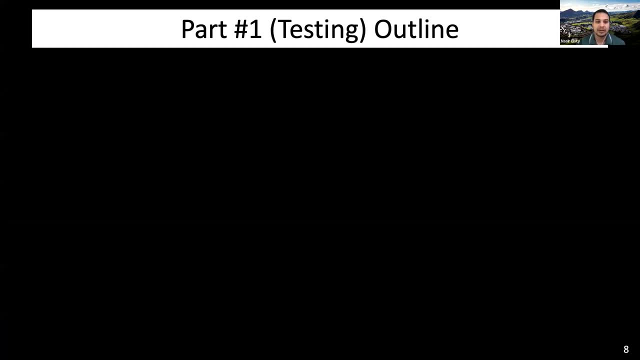 using a tool called NVivo. Then we find out the discrepancies, sat together, discussed and decided the final results. So in this first part of this talk I'm going to discuss the demographics of the participants and then what level of knowledge. 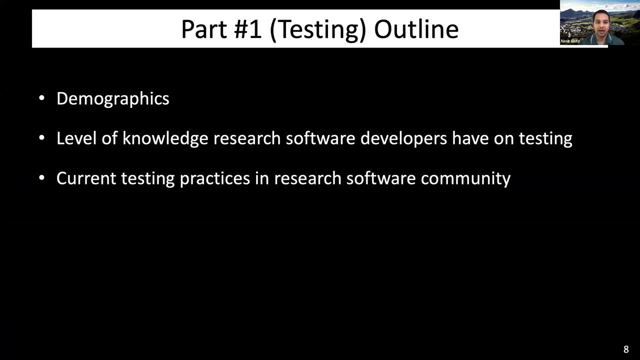 do research software developers have on testing? Then how do research software developers test their software, And why is testing research software difficult? And is it possible to adapt existing testing techniques to test research software? And what improvements to the testing process do research software developers need? So at first, demographics. 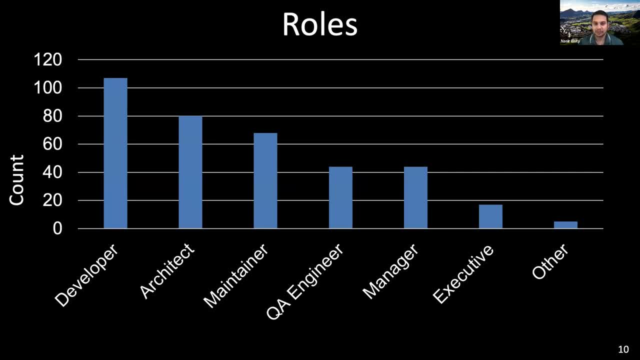 So developers' project role could affect their perception of testing. So identifying and the distribution of respondents' role also helps us judge whether the survey reached a broad and diverse set of research software developers. This figure shows the respondents were skewed more toward technical roles. 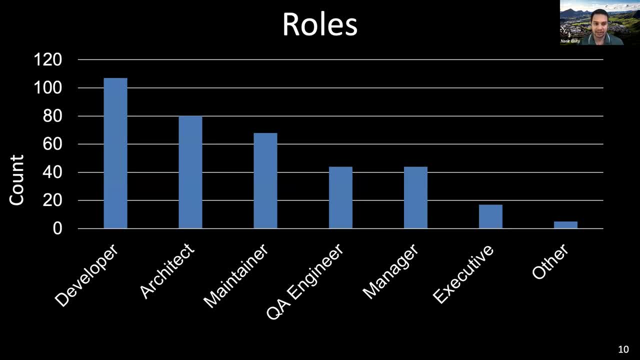 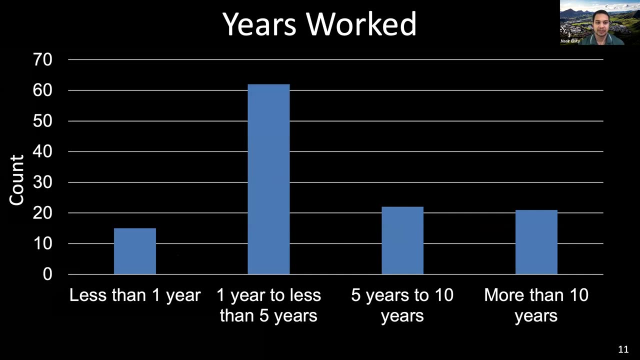 that is, developer and architecture, and then towards non-technical role. Something to notice here: because the respondents could choose more than one role, the total in the figure is larger than the total of the responses. So, for example, if you put a 3-year experience in a research software, 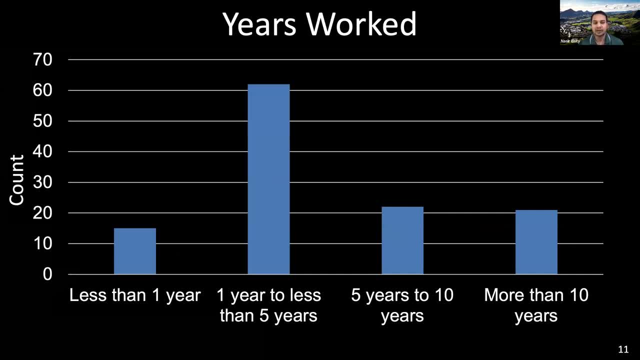 the range of the responses would be 5 years, to be an average of a year, rendering the survey a class of 10, which is the same as the data from the survey, Which results in a small increase in response in terms of the responses. 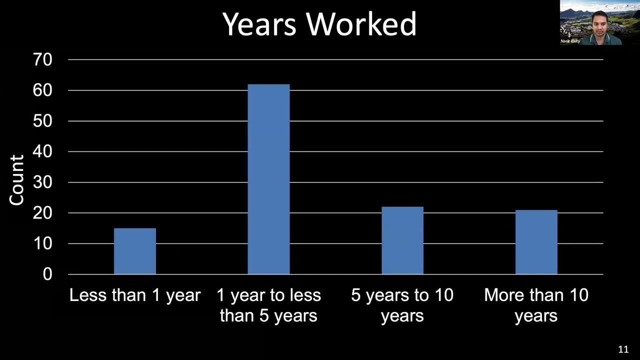 which result in a less than 1 year of experience in a research software. So this figure indicates that most participants had more than a year of experience working in research software And just under one third had more than five years of experience, and only a small number had less than one year. So this distribution suggests that the number of respondents 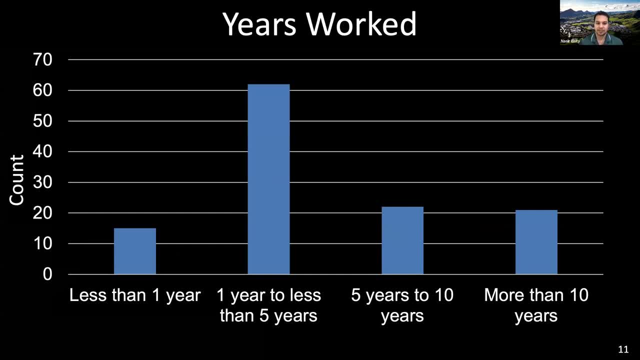 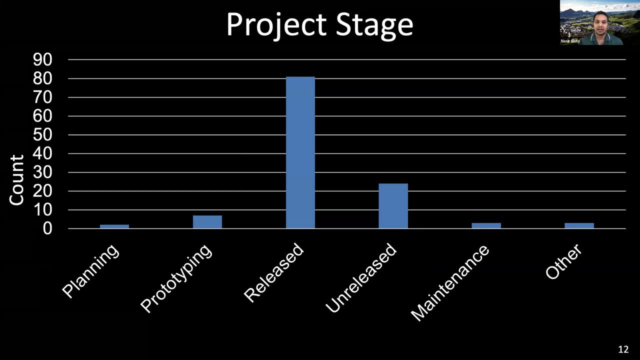 that the participants had appropriate knowledge and experience to provide valid answers to the question. The project stage helps determine which types of testing may be most useful. The projects represented by the respondents were overwhelmingly in the released state. This result is important because projects at this stage should have already established. 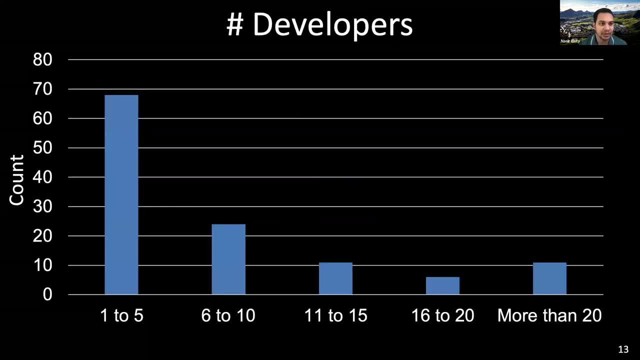 testing programs that they deem useful And number of developers. So, because teams of different sizes may have different perspective on the use of software engineering practices, we asked the respondents about their project size And we can see in this figure that most of the respondents worked. 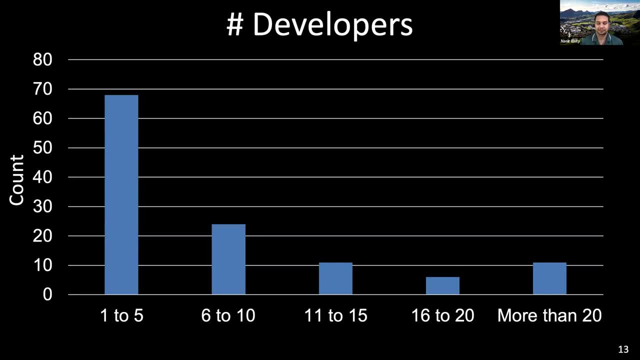 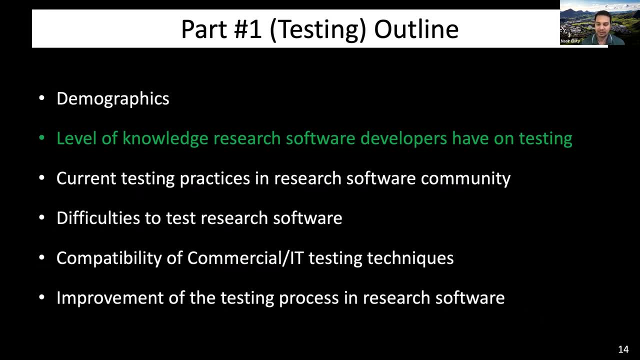 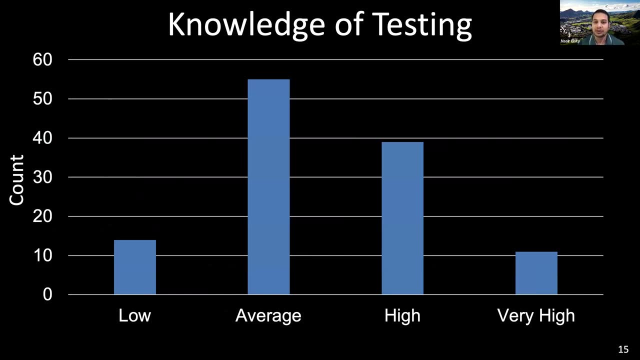 on smaller teams in terms of number of developers. So what level of knowledge do research scientists have in terms of the number of developers? What level of knowledge do software developers have on testing? We asked the respondents in a survey question that: how confident are you on your knowledge? 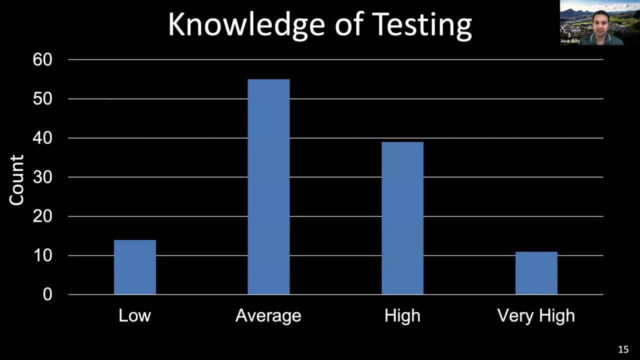 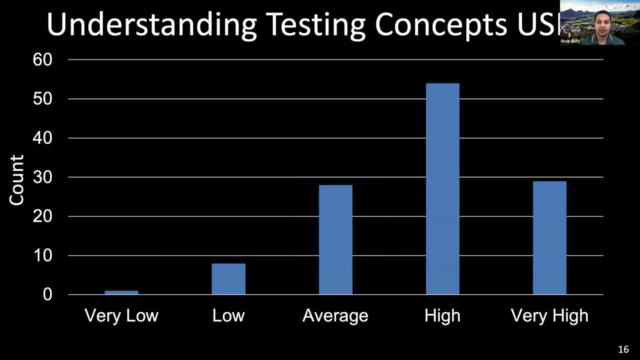 of software testing. So most of the respondents mentioned at least average level of confidence, of knowledge of testing, And more than one-third respondents saying that their confidence level is in the range of high or very high. While we asked their understanding of the testing concept used in their project, more than half of the respondents mentioned high or very high. 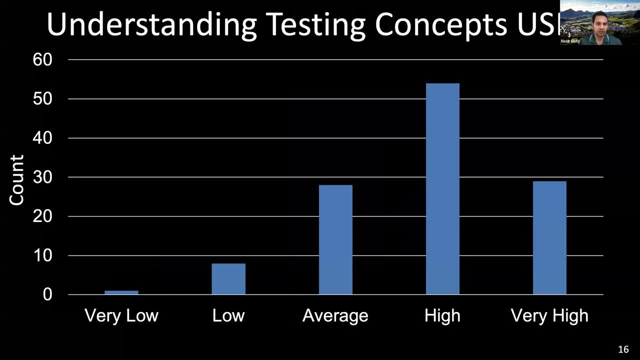 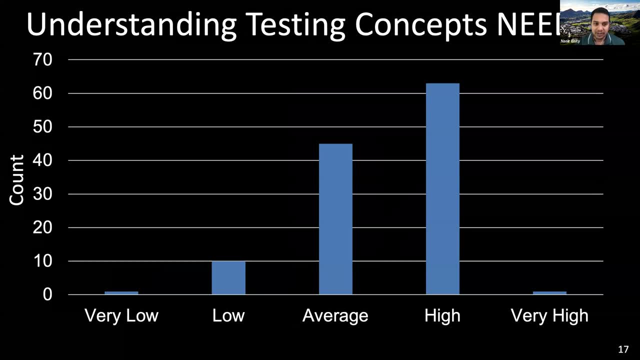 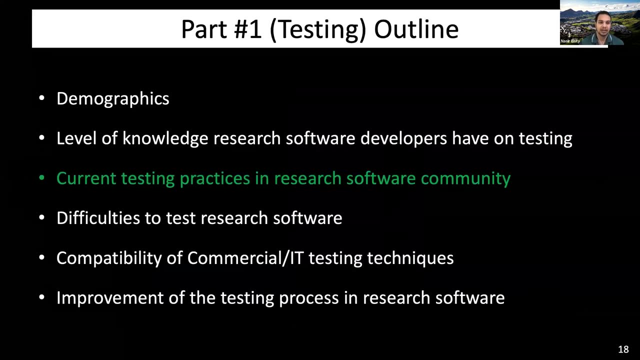 understanding, And only a few participants mentioned low or very low. And in terms of the understanding of the testing concepts needed in their project, the respondents are over. the responses are overwhelmingly in the range of average and high. Now the question is: how do research software developers perform testing? 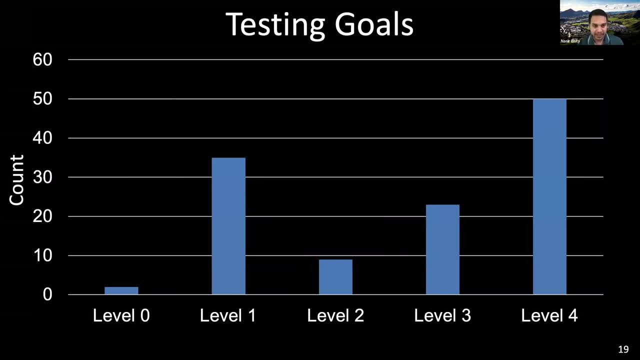 We asked the respondents about their testing goals And these goals are standard testing goals and we inherited these from the software testing books of Paul Amon. So maximum number of the participant mentioned level four. So, which means testing is a mental discipline that helps all researchers develop higher quality. 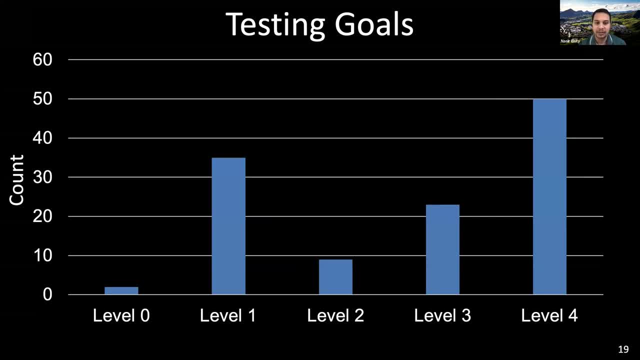 software And the second highest number of participants indicated level one, which means the purpose of testing is to show correctness. The next highest level is level three, which means the purpose of testing is not to provide anything but reduce the risk of using the software. Just so you know, level zero means there is no difference between testing and debugging. 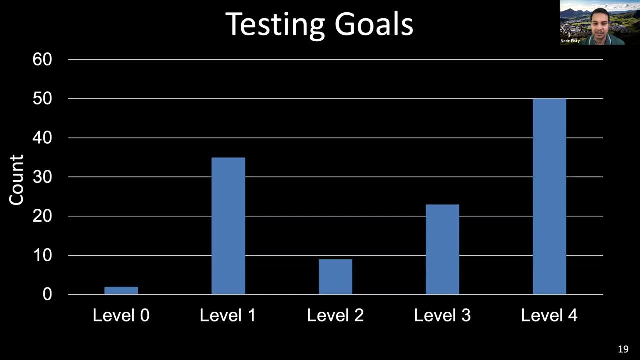 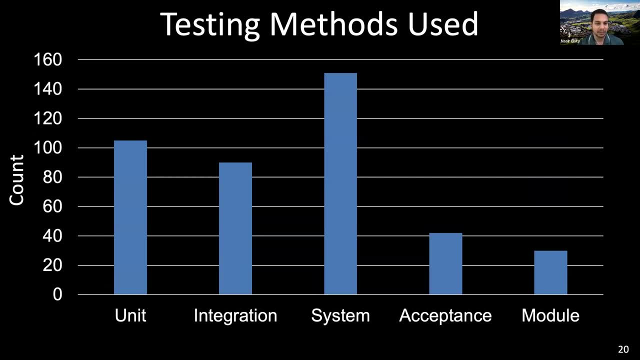 and level two means the purpose of testing is to show that the software does not work. Then we asked the respondents about their usage of testing methods. So system testing is the most popular one in research software development And a lot of the respondents mentioned unit and integration testing as well. 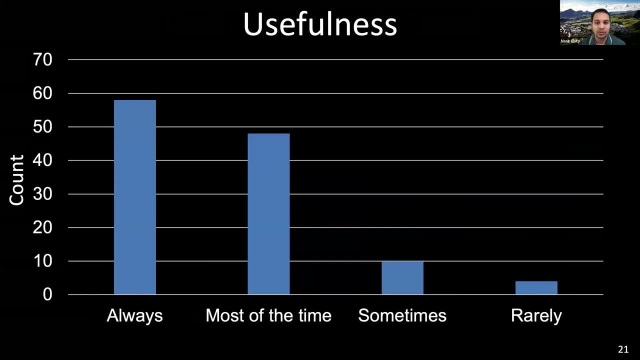 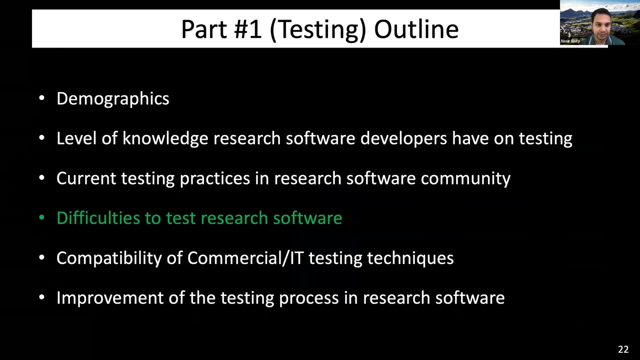 So, in terms of usefulness of testing, almost all of the respondents mentioned testing was useful always or most of the time. Only few participants mentioned sometimes and rarely, and no one mentioned never. That was another option. So why is testing research software difficult? 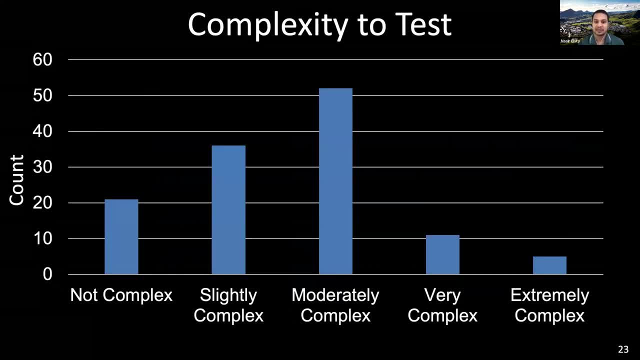 So we asked the respondents that how complex is their testing process? So we can see in this figure that half of the respondents indicated at least moderately complex to test their project And one third of the participants mentioned slightly complex. Then we asked them to explain any challenges or barriers they face to test the software. 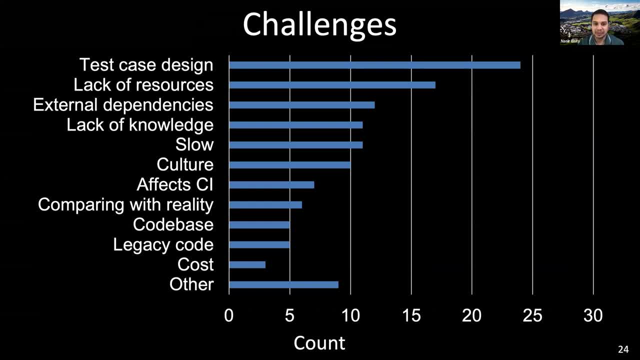 So we asked them to explain any challenges or barriers they face to test the software. So we asked them to explain any challenges or barriers they face to test the software. The most common answer to this question was test case design. So because application cases are usually too big or expensive to test, 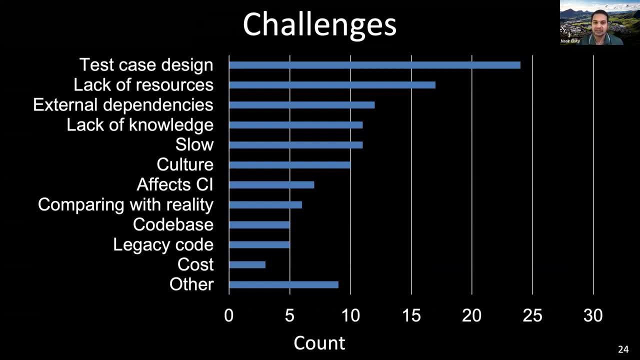 so breaking them down to meaningful system tests is a challenge. And the second most common answer was lack of resources, which means lack of money, lack of people or lack of time. The next thing is external dependencies, Which means research software often depends on external hardware. 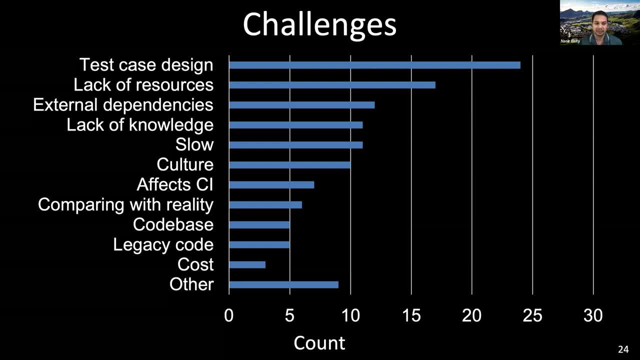 software compiler, et cetera. that makes testing difficult And because research software developers are not trained software engineers, so there is always a lack of knowledge And many respondents found their testing process is very slow, but they always have some sort of deadline to finish the task. 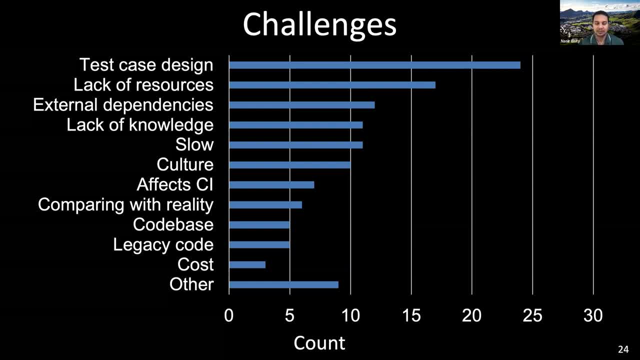 So there is a cultural difference between the researchers and the software engineering community, And one unique challenge research software developers poses regarding testing is comparing with the reality. That means testing ocean model or climate control or nuclear weapons or something like this, And because of the lack of proper knowledge and resources. 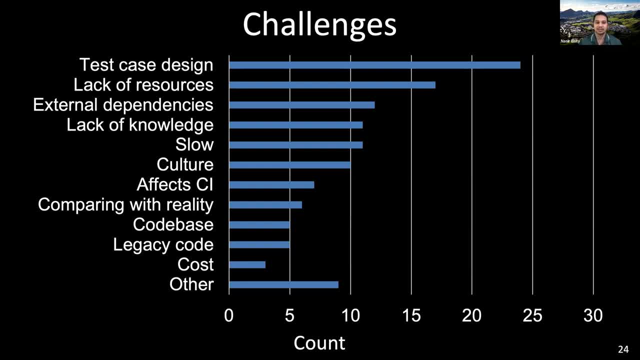 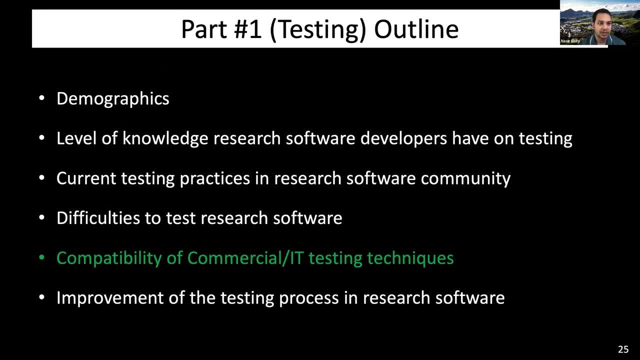 they usually have a poor code base which is hard to test, and many of their code is legacy code. Also, there are a few other challenges as well, So I'm going to start with the first one. So in this case, 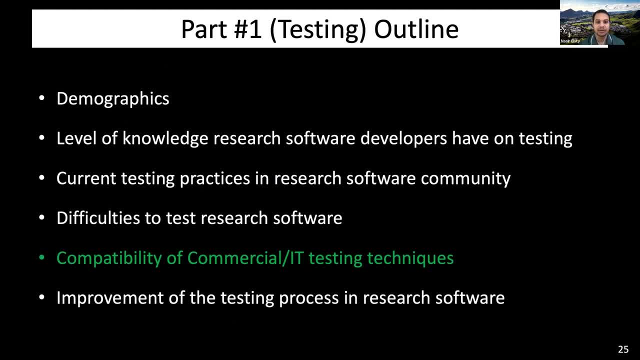 the compatibility of commercial IT testing techniques. we refer to the testing methods currently used in commercial IT software development, And these methods include unit testing, integration testing, system testing, acceptance testing and module testing, And gaining a better understanding of how these methods apply to the testing of research software. 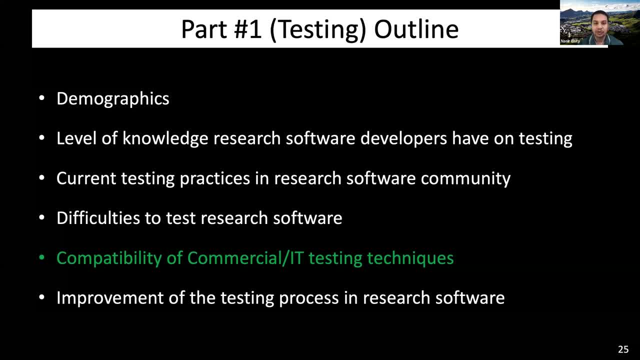 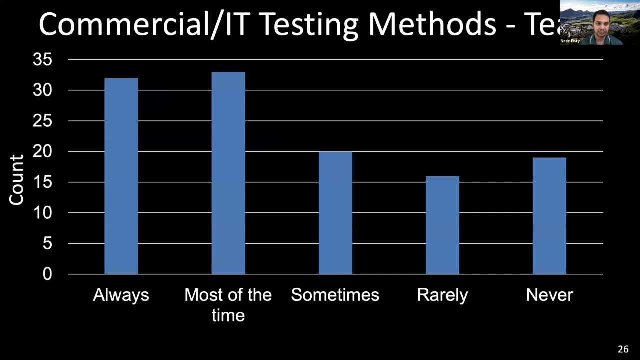 will help research software developers have more confidence in the methods they use and reduce the need to discover this information on their own. So we begin with the survey question about the frequency with which respondents use commercial IT methods as a team. So, as this figure shows, most teams apply this method, at least sometimes. 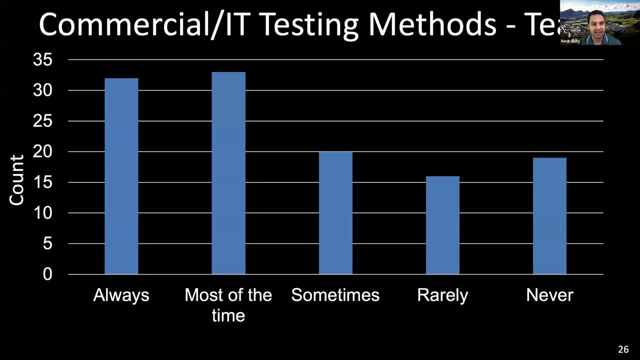 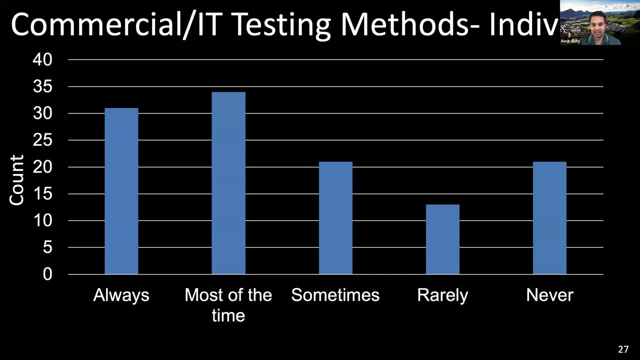 And there are a few teams that apply commercial IT tests rarely or never. Similar is the case when we ask the respondents whether they use commercial IT testing methods personally. So, as this figure shows, most individuals apply these methods at least sometimes, And there are a few individuals that apply commercial IT tests rarely or never. 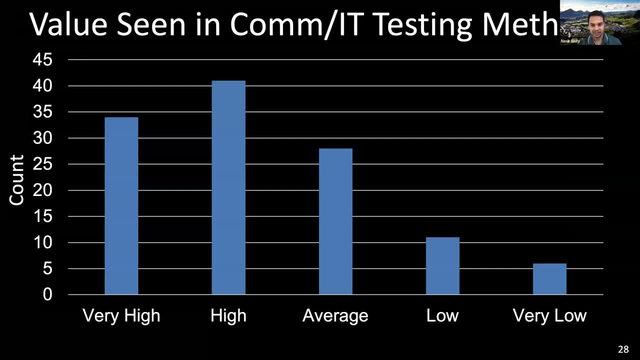 So, beyond whether the respondents use the commercial IT testing methods, we ask the level of value they see personally in using these methods. The distribution of these results in the figure we can see is: The distribution of these results in the figure we can see is: 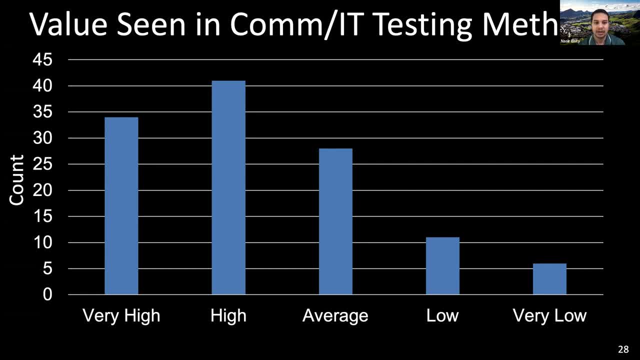 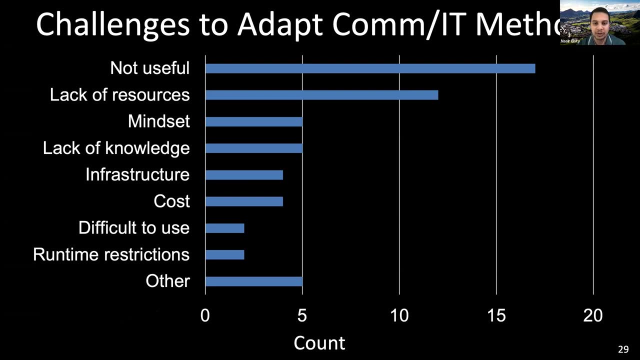 that respondents generally saw a value in using such methods, and with more than half answering high or very high. To gain an insight into where the commercial IT methods cause problems, we asked the respondents to explain any challenges they face in an open-ended manner. 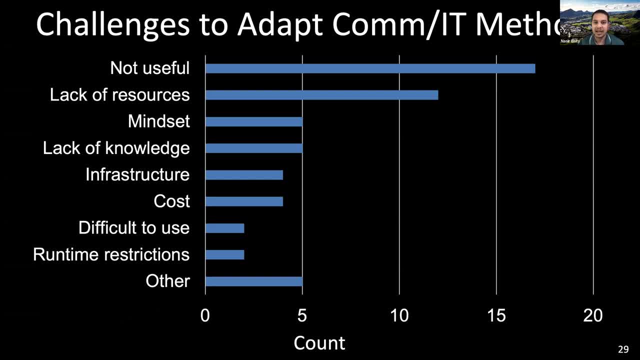 So our qualitative analysis of the results identified nine high-level categories of challenges. So our qualitative analysis of the results identified nine high-level categories of challenges shown in this figure. I discussed some of these challenges in detail in response to other questions, so I only highlight a subset here. 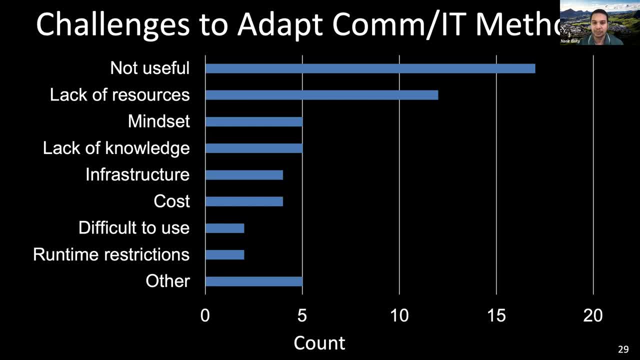 Overwhelmingly the most common challenge respondents reported was that the methods were not useful, And this challenge arises because research software is typically not production software and some commercial tools do not account for the issues with numerical tolerances, And it is difficult to adopt a commercial idea. 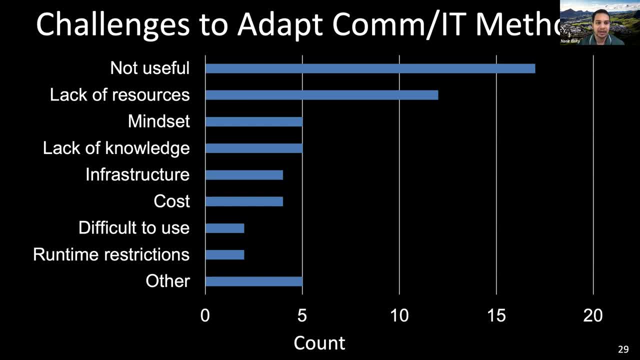 but this is one of the most common challenges. Want to discuss a few examples That are quite similar to the overall overall difficulties with testing well-designed research. So there are two different kinds of challenges. One of them is the lack of information where we're taking these knowledge from the commercial IT testing methods through the development of 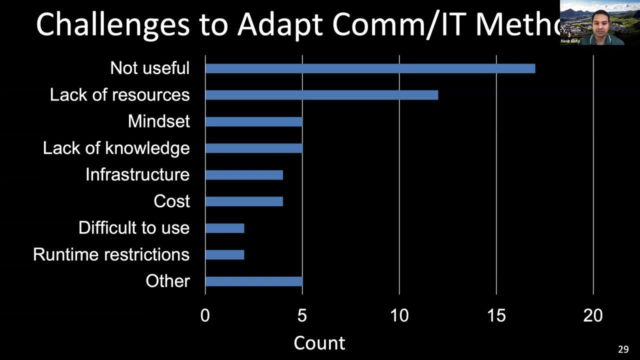 scientific software because of numerical errors and often not knowing the expected output And similar to the overall difficulties with testing research software. The second most common challenge is to using commercial testing method is lack of resources, And one respondent explained that the challenge as lack of expertise, schedule demand. 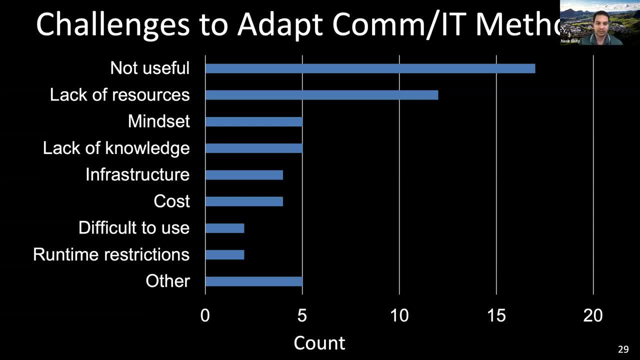 lack of R&D and software development-oriented tools, etc. The third most common response is the mindset of the research software developers. The problem is, the developers often feel like any time not spent developing code for the core software is not real work, and thus time spent writing tests is less enjoyable. 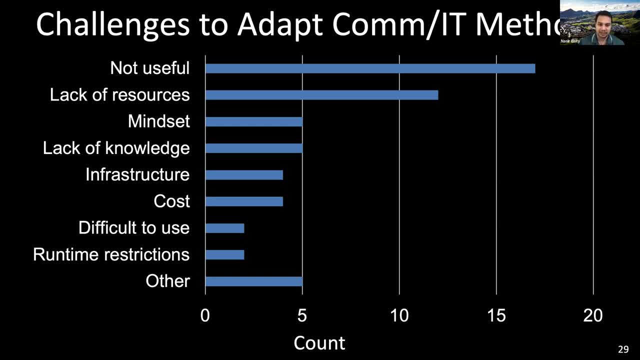 In addition, the problem is cultural. That means convincing people that it is beneficial, necessary and worth their time and not insulting to their work. There are also challenges with mindset that originate external to the team, such as the funding agencies are generally not aware of their importance and effort spent on testing. 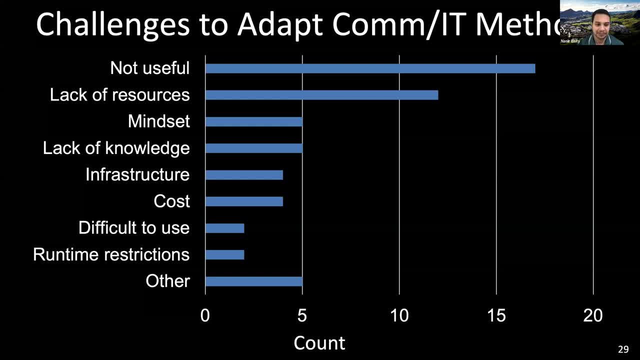 is effort not spent writing or publishing papers. Finally, there is a lack of family engagement. The problem is that there is no similarity with the ensemble of testing patterns and goals available. Moreover, there is a lack of knowledge need for infrastructure support, expensive or difficult. 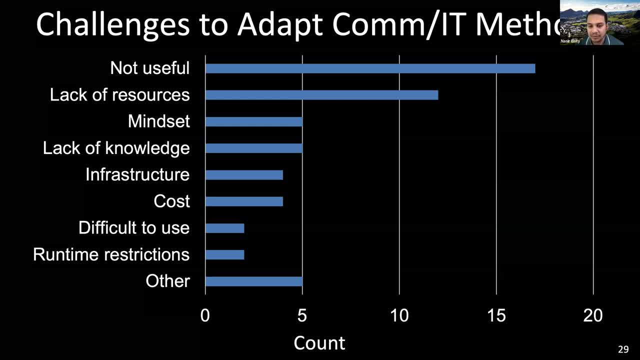 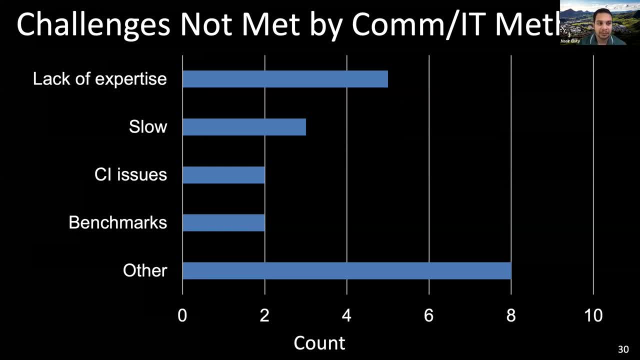 to use and runtime restrictions. that makes research software difficult to adopt. commercial IT testing methods- Challenges not made by the commercial IT testing methods. There are cases where the methods do not meet the needs of the research software developers. These methods are just not applicable. 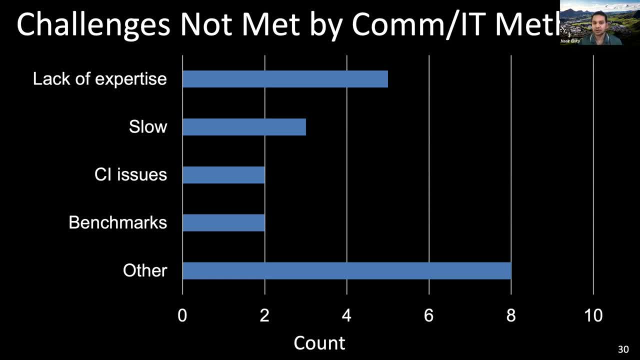 So we asked the respondents to explain any challenges that could not be made by commercial IT testing methods. The quantitative analysis produced five high level categories of challenges. we can see in this figure. The most common challenge, by a large margin, was that the methods do not meet the specific needs. 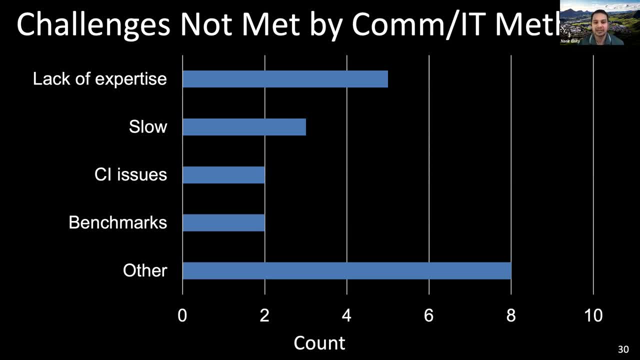 of research software. These specific needs can include visualization, image processing and analysis, fluid flow simulation or simulations where there is no analytic solution or known correct answer. that means no oracle. So a unique challenge of research software is that validation requires domain expertise. 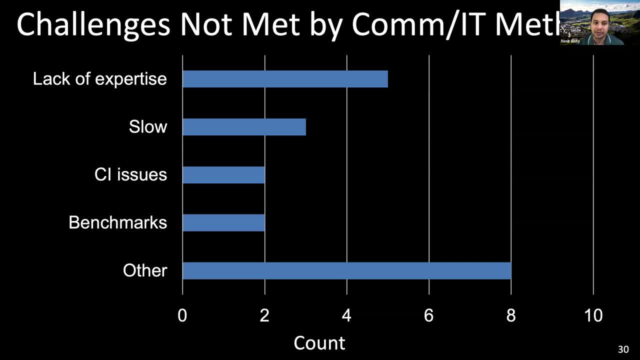 which is sometimes difficult to express in the commercial methods. And another situation that is common in research software is whether the results are meaningful, as it is. respondent stated, IT methods are good for preventing errors but not good at catching if numbers are no longer meaningful. 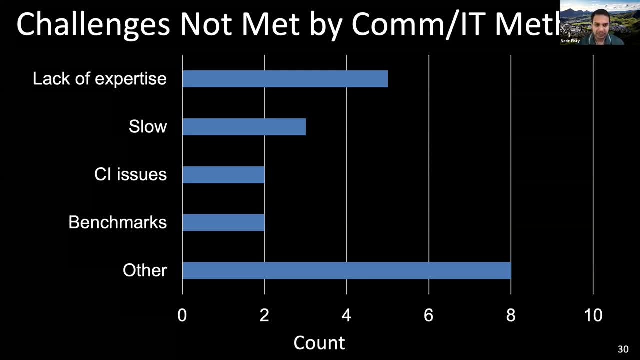 or charging to determine. So the respondents also mentioned a lack of expertise, slow to execute the test and continuous integration issues and benchmarks as some of the challenges and that could not meet the commercial IT methods And their decision, because the data needs to be. 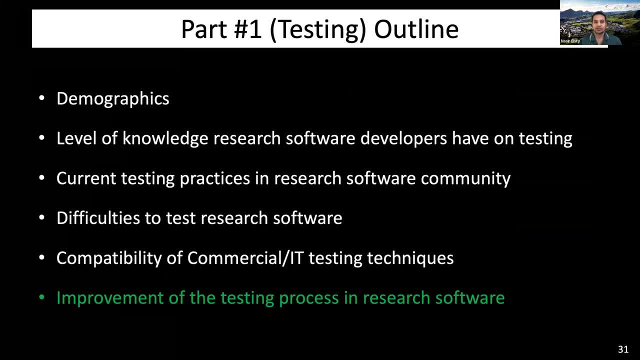 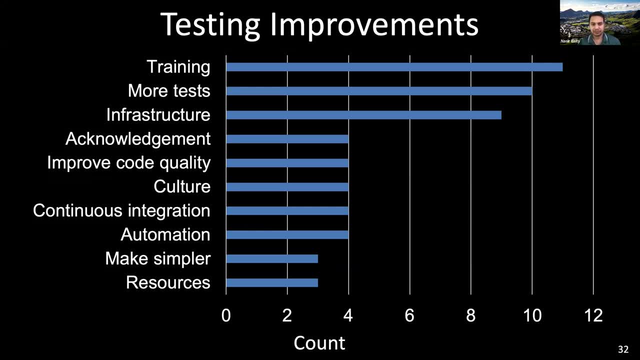 longer to be able to understand and understand publicly. So what improvements to the testing process do research software developers need? In terms of the improving the testing process, respondents mentioned there is a need for training, such as education, examples, templates, so that they can use proper testing methods. 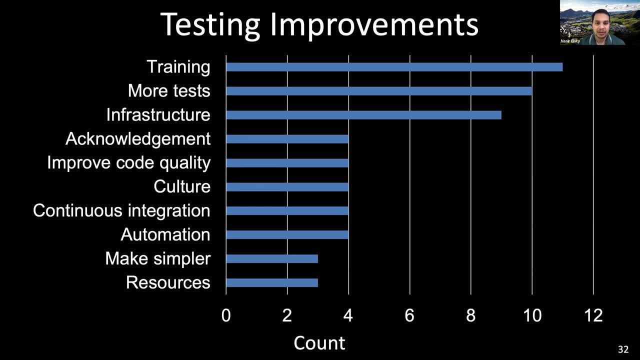 And they also mentioned they need more types of tests and infrastructure support. that will cover the tests and infrastructure support And in addition, they also mentioned that there is an increased over specific needs of the research software. And another important aspect is acknowledgement. 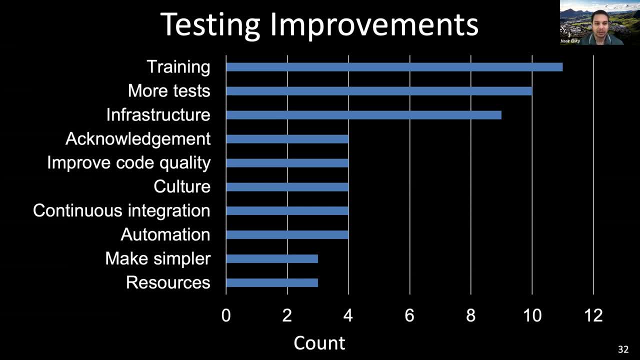 for their time and effort is spent on testing, And respondents also mentioned to create a culture of testing in the research software developers community. that will help improve code quality and continuous integration. Moreover, making the testing process simpler and enough resources can potentially improve the testing process in research software. 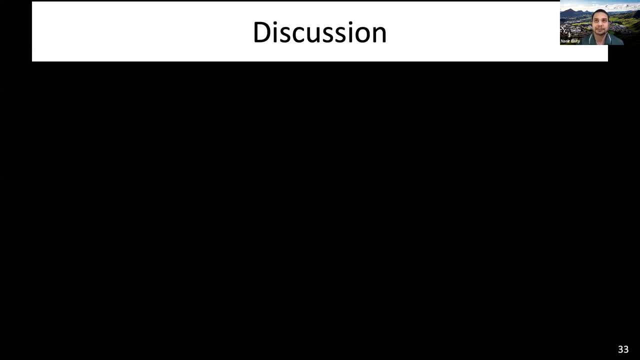 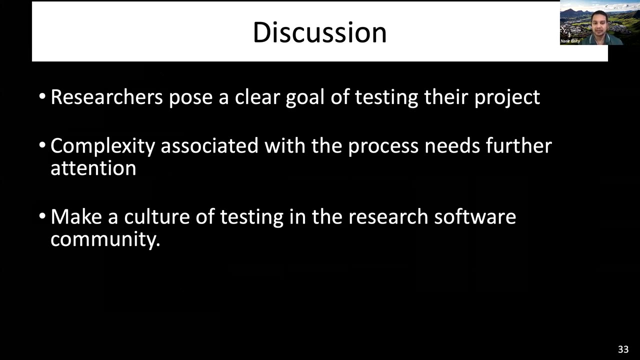 So, to wrap up the first part of this talk, overall researchers pose a clear goal on testing their project, but the complexity associated with the process need further attention. to make a culture of testing in the research software community and providing proper training and resources can potentially improve the testing process. 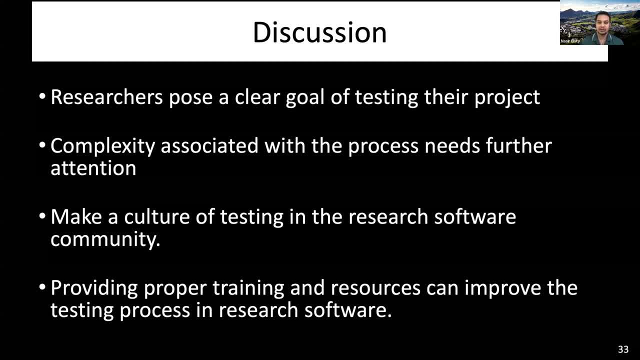 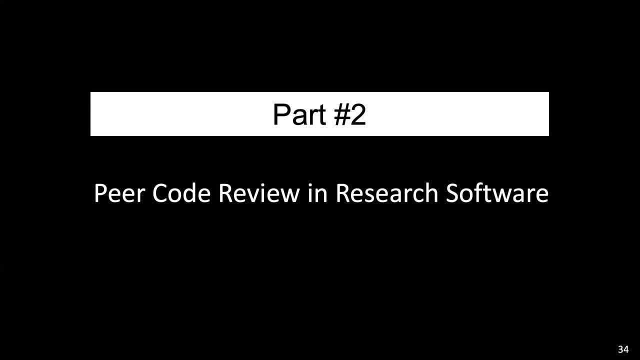 in research software. So thank you again for your time. I am jumping into the, So I'm going to pause you for a second Marsha, because we have some questions from the community about this first part. OK, David, do you want to go ahead and read the question? 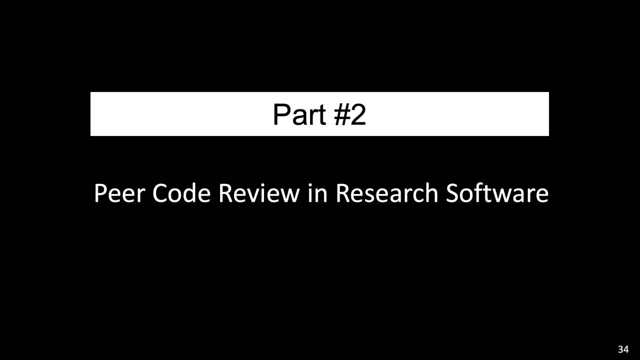 Yes, So I just posted again the link to the Q&A document And if you go over there we'll see four questions. One: Do you think the lower-end testing factor will be better? emphasis on quality with research software is due to people not knowing. 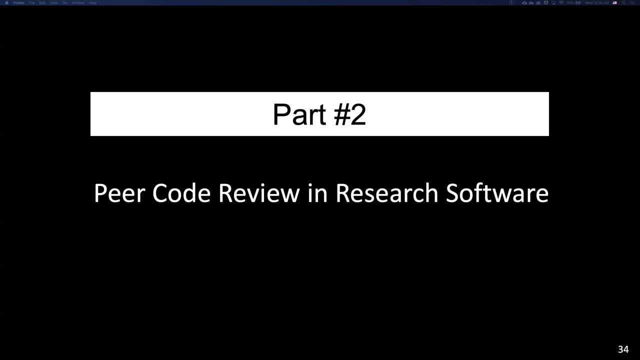 software community not well trained enough or something else? I think both- yeah, people are not trained enough or not well trained enough, and also the motivations to do the testing. so while working on on the testing, I worked on the Los Alamos National Laboratory. so the people I worked on, they were sincere. 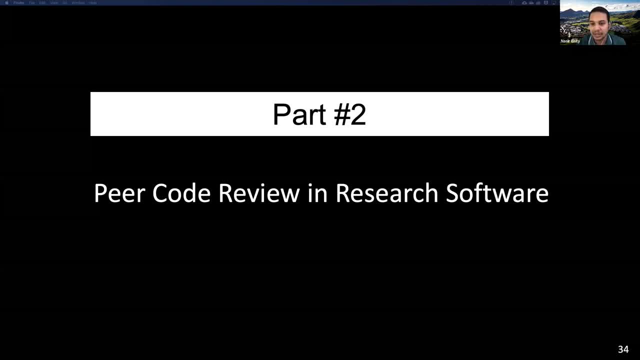 but I talked with many people in the in that laboratory that and they think testing is useful but they don't have time to do that and and they don't have funding and they don't have the motivations actually to work on testing and but but people think this is necessary. that's the good thing, and if 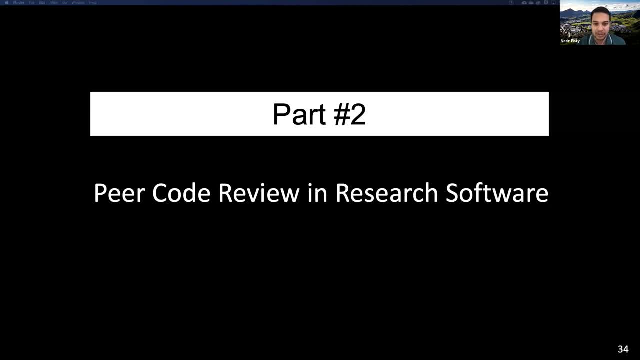 we look at the papers that were published, like if three or five years ago and people mentioned that they don't see the next phase of testing and they don't have time to do that and they don't have necessity or they don't feel the necessity. so nowadays things are getting. 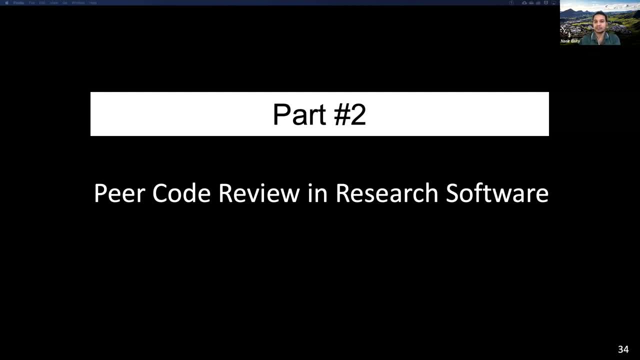 better and people are more into adopting software engineering concepts, especially testing, code review or any other software quality practices in research software. so, yeah, things are getting better, and also the BSSW initiative and there are research software engineering groups that are helping with improvement of software engineering practices in research software. okay, next question: how do we? 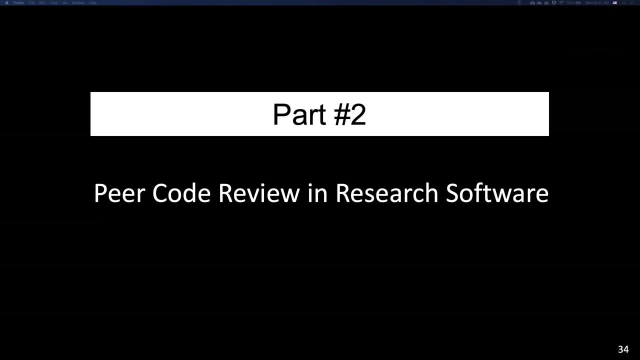 ensure software quality without intervening with research and frequent changes to the software, especially if researchers are developing the software? how do we ensure software quality without intervening in research, maybe? I think maybe the question is trying to ask: you know, because research software is, there's a lot of frequent changes, of course, and that how do you? 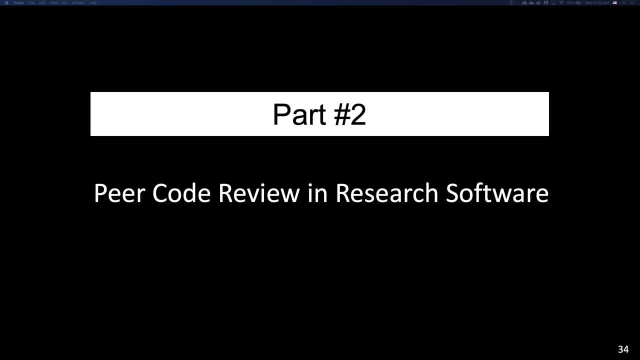 not impede the research but still ensure software quality. so they're competing interest. yeah, that's why a system testing would be better, because research software changes frequently and so if you want to test everything but in after every iteration of the changes, it may be difficult to. 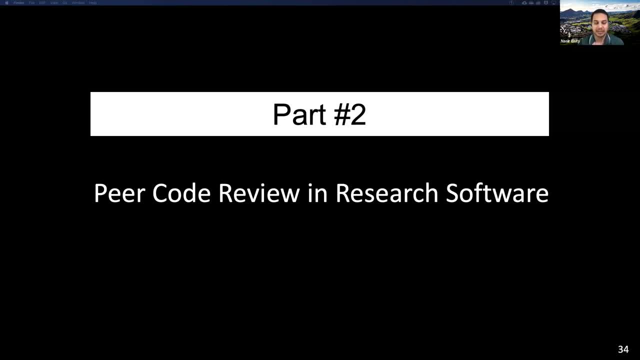 write another test. so there are two things. one could be the test, even development, so you develop the test first and then develop the software so that you already know what are the things you are going to develop, or you do the test at the end, so you you have your module in a stable state first and then 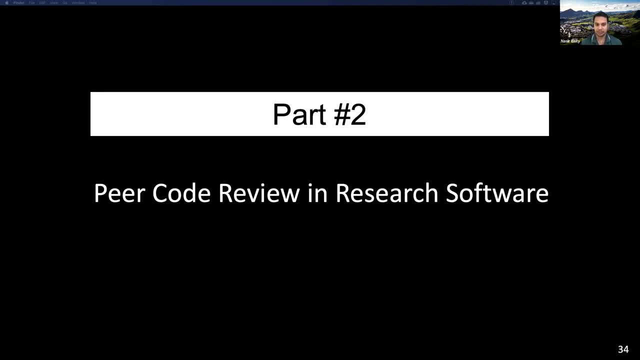 you jump into the testing process. so both works, but it depends actually on the actual software or actual research associated with, because underlying science is the difficult part. on software testing in research software that usually doesn't have in the quality commercial or IT software. yeah, okay, so I'm sure you've gone to the next question. yeah, do you differentiate in? 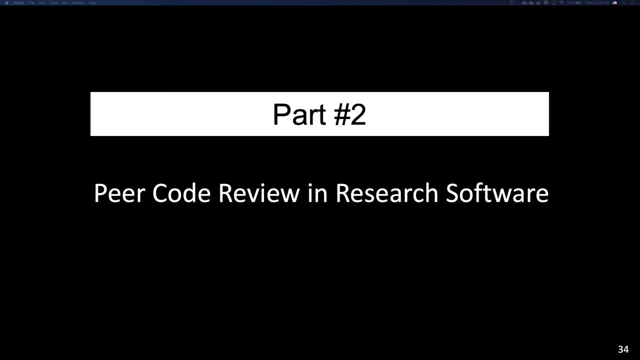 any way between automated and manual testing. yeah, there is this. this is different, so you can do both or you can do one. so it depends on which your project actually and and the the timeline you have or the project goals you have. so for some projects I know that, so you. 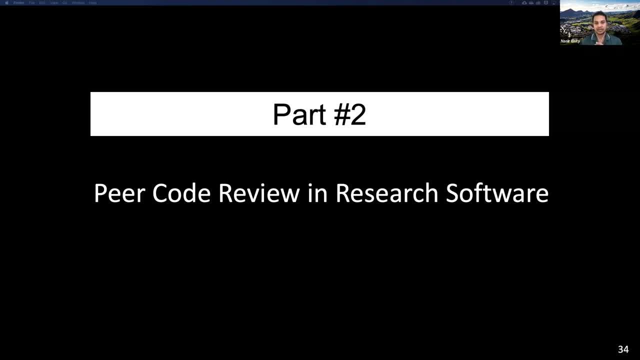 have the specifications. you have the specifications that you have to do those things. but that doesn't apply to manual testing, because manual testing is not the way to go. the automatic testing is not possible because there are some adjustments after every iteration and I have seen some research software there. 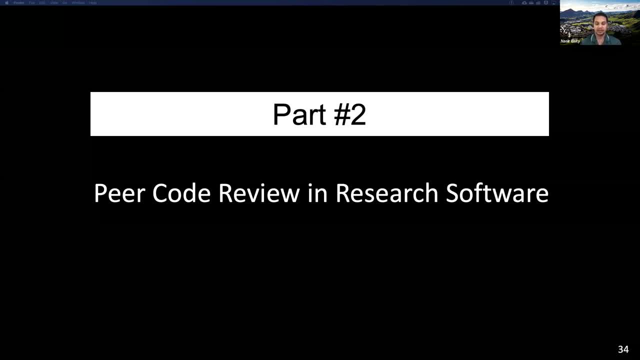 iterate over a month and then finally produce a software test. so and if that output changes in the next iteration? so it is difficult to employ automated integration system. but yeah, so there are differences and i think it depends on the projects and many of the software engineering questions are. it depends, because every project is different and every project. 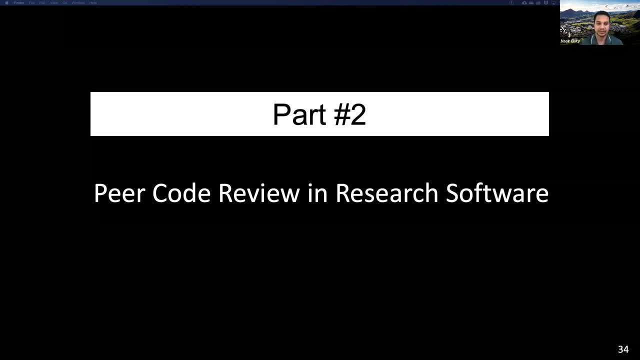 has different characteristics. yeah, the next question. oh yeah, sorry, yeah. well, i think that question about the automated testing and manual testing also refers to your survey results as well. was there any sort of differentiation between automated testing versus manual testing in your? oh? so we didn't differentiate that in. 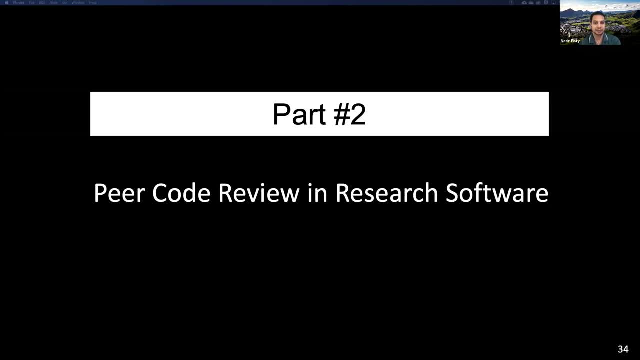 the in the survey. yeah, so people did not explicitly mention that what kind of testing they are doing, but we are doing a follow-up survey and some for in-depth results of the, because this survey is the preliminary survey. so this is step one and now we are moving further to. 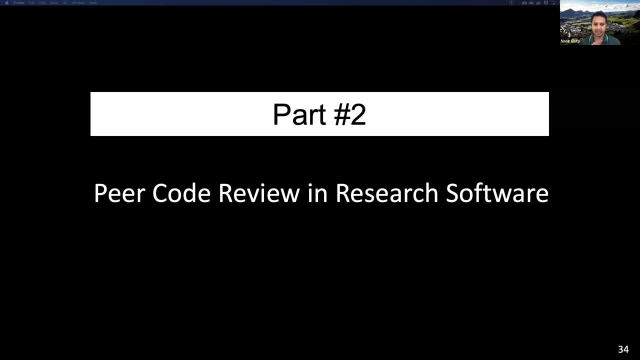 step two and then, finally, we will try to develop some testing techniques that will directly, uh, help the research software community. so we are trying to go in depth on the next step and i think i hope to find something for my clarification. i'm kind of reading this question. 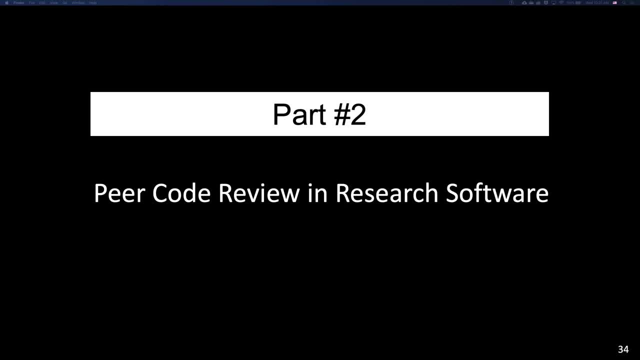 i want to be sure that we- i don't think that if you're- if you're running the code and looking at a number and writing a number in a spreadsheet or reporting a result by email, that that counts as as testing. so all testing should be somewhat automated in the sense that there is a command. 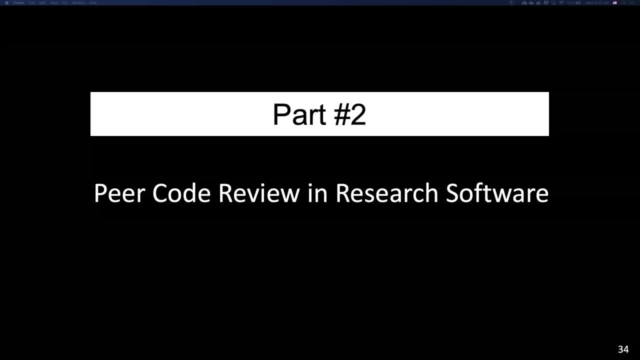 whose purpose is to give you a true false yeah, yeah, that's the purpose of automated testing, but in many cases, you don't have the answer, so you may have to use your expertise. like you, you know the science or you know the algorithm- that it might look like this. 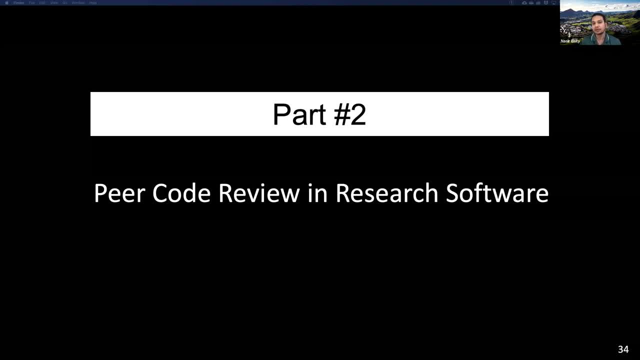 or you might produce a graph that you might have to- uh, you may have to, like do some assumption that, yeah, this might look correct. so this is not the usual case, but this may in some cases where people do manual testing, but yeah, but it is recommended to do automatic testing, so that 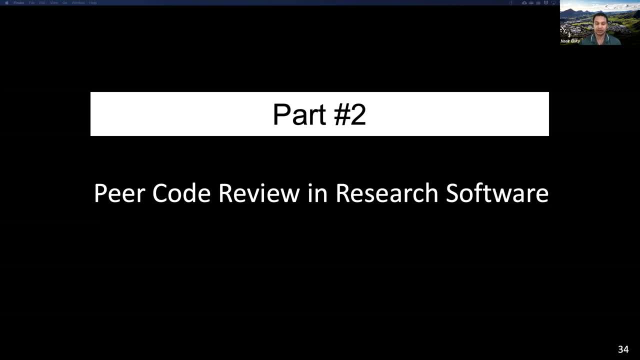 you use some statistics, even if you don't have exact output or anything, so that you can get some yes or no from your continuous integration system. okay, and i'm gonna read just um this next one here, and i don't know how much time we have for questions. 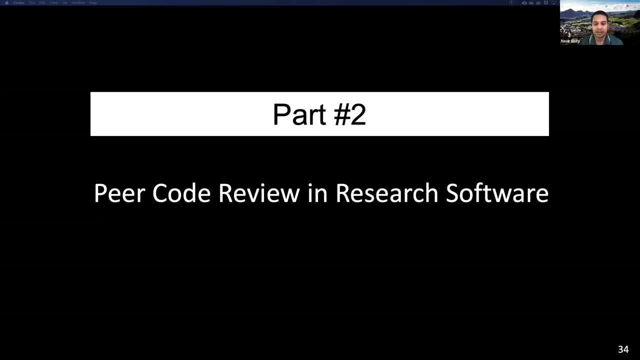 before i move on to the second part, we can come back to the questions after the talk, i guess. yeah, yeah, so the next one might actually get a little bit more in detail. um, decide if you want to answer this one. what do you want? what do you classify as? 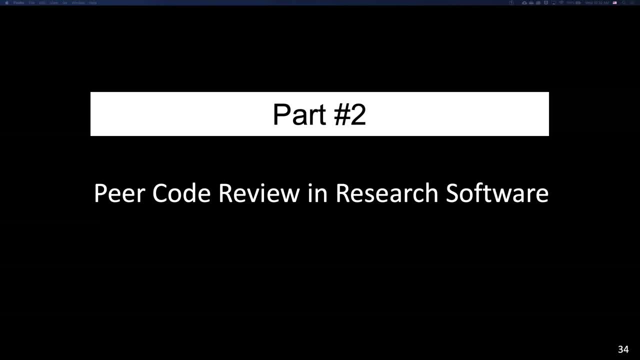 commercial testing methods. does that include cicd or fuzzing, and did you provide a definition to the participants? maybe if you just answered the second part of that question then we can move on with the talk. yeah, and i'm going to the question. so there is two things. one is testing method and one is 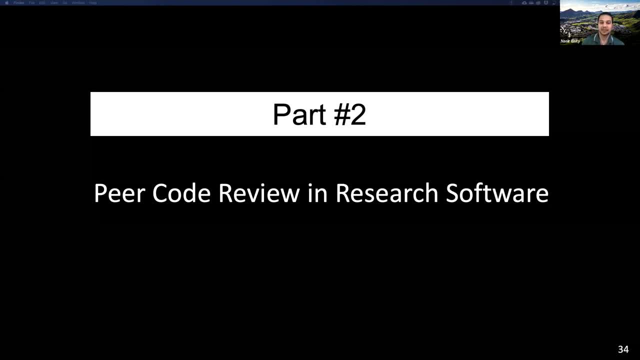 testing technique. so testing methods are the methods like unit test or or system test. integration test and testing techniques could be the more in general items like fuzzing testing or boundary values testing or any kind of testing like metamorphic testing or runtime assertions. so these kind of 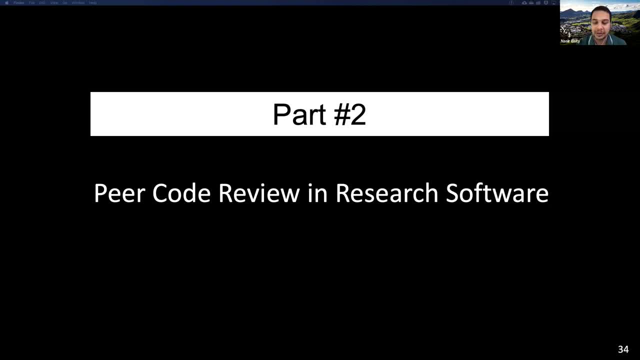 things. so we provided every definitions in the uh survey. so we clearly mentioned which is methods and so, so that everyone can be in the same page, we- uh, we provided definitions of the testing methods and in some questions we have like 15 or more testing techniques and so we define all of them and even if uh. 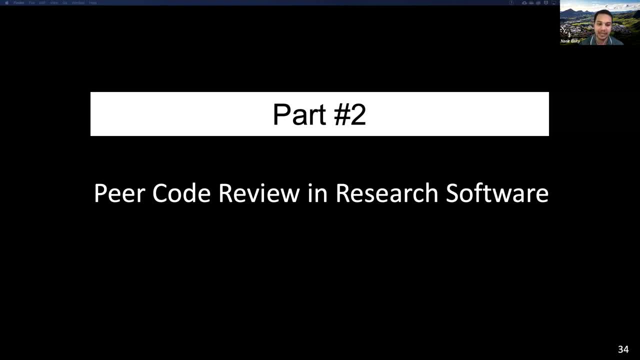 when we say commercial id testing techniques, we also define that so that people are in same page. because i know we have different kind of definitions in our mind and there is a paper you can look in online that how many definitions are there on unit testing. so people have their own kind of definitions in their 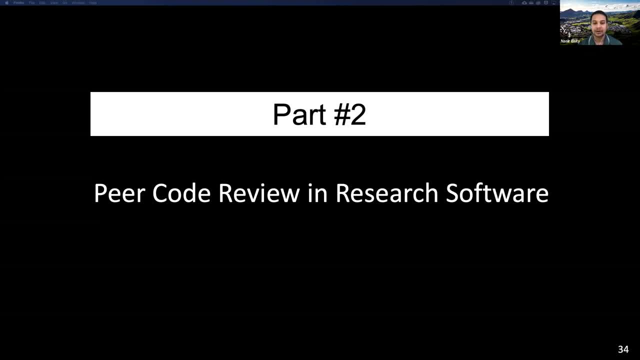 mind, so bringing them into one unified platform. we provided definitions and we piloted the survey with uh prior spreading it out, so that this is understandable. yeah, all right, thanks, maybe we can go to the presentation now, or? yeah, we'll pay the questions you want to answer. go ahead. 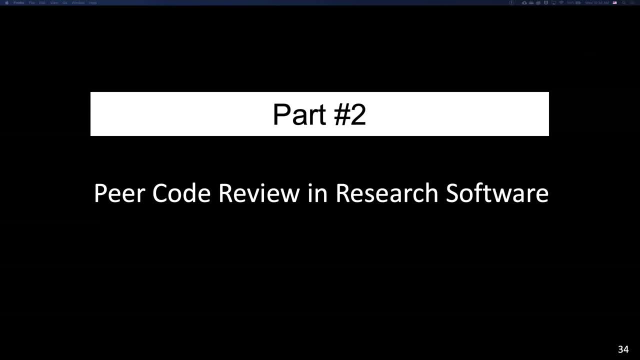 otherwise i think we should probably continue any thoughts. i agree, why don't you go ahead and continue with the pure code review? yeah, then we can come back to the questions. so you can still see my uh screen right? yeah, okay, i just wanted to make sure, because there was the browser and the screen, all that, okay. 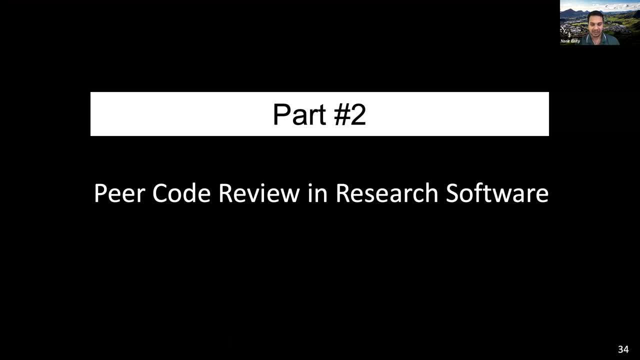 yeah, so, yeah, um so, uh, uh, the first part. we discussed that research software has complex computational behavior. so this complexity, along with the fact that the expected output are often unknown and makes it difficult to test research software. so in many cases the input space of research software is so vast that it is not feasible or even possible to develop a test suite to remit. 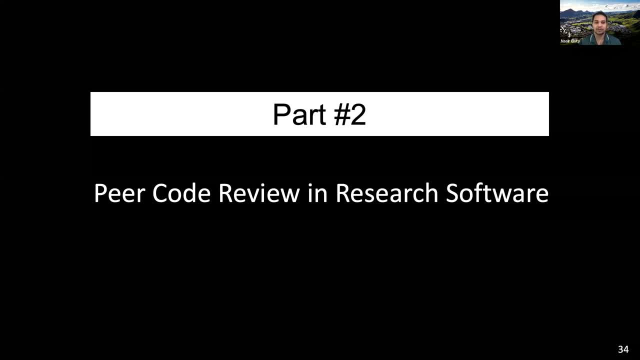 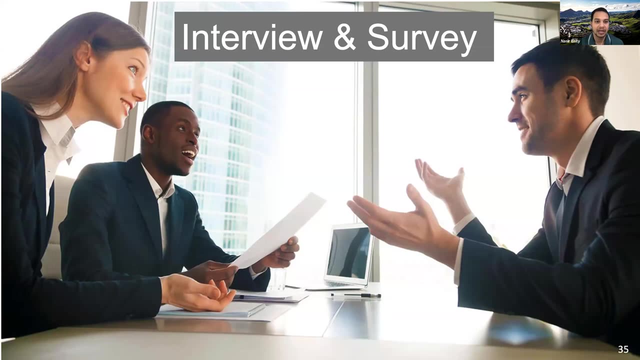 this situation. a code review is a systematic examination of computer source code by other peer and remove vulnerabilities and code reviews recognized as a beneficial tool for improving software quality. so for this study we gather data from two sources: interviews and surveys. so we first enumerated and overall research. 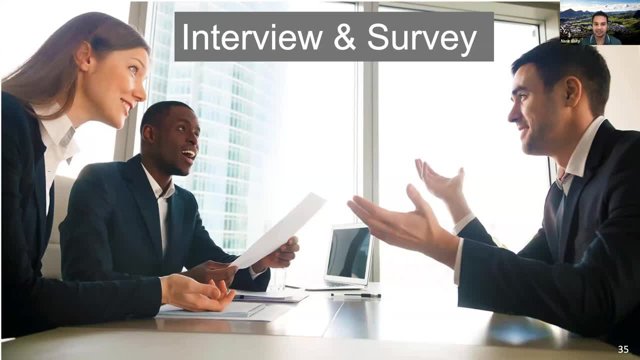 questions and based on the research questions, we then identified a series of specific survey and interview questions and as part of internship at the National Center for supercomputing applications and CSA, I had the first hand access to research software developers to conduct the interviews and after that, to reach a broader audience, we can conducted a Sun survey. so we 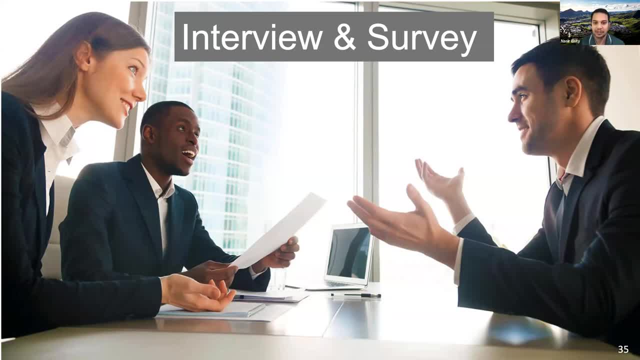 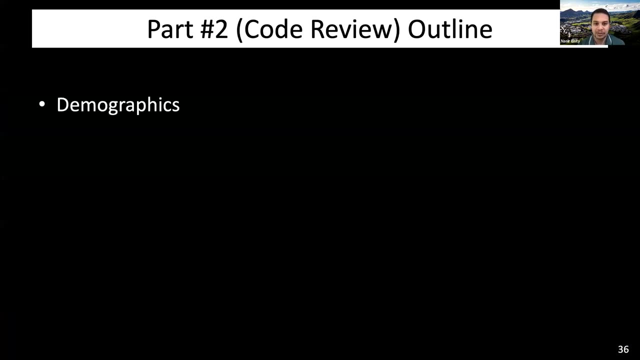 included 22 interviews and 62 server responses to this study, and the participants were from more than 50 projects and all of them had at least some experience with code review. so, similar to the first part, I am going to describe demographics of the interviewees and service. 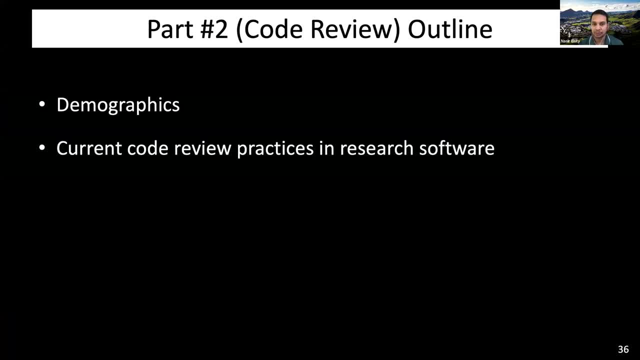 respondents and then I will discuss: how do research software developers perform code review and what effects does code review have on research software and what difficulties do research software developers face with code review and what improvements to the code review process to research software developers need? yes, at first, the demographics. so number of years work on research software, so this: 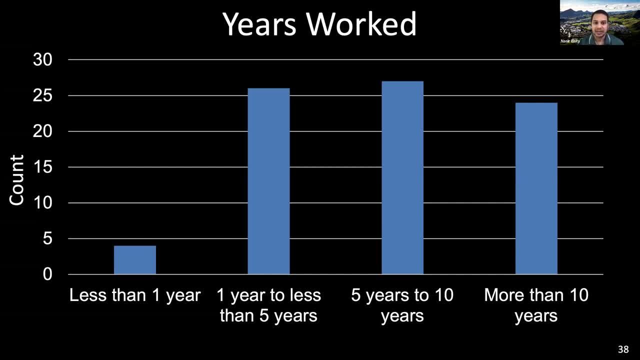 distribution of respondents indicates most participants had at least five years of experience working in research software and just under one-third had more than ten years of experiences and only a small number had less than one year. so this distributions are just that participants had appropriate experience and knowledge to provide valid answers to the questions. and yeah, a. 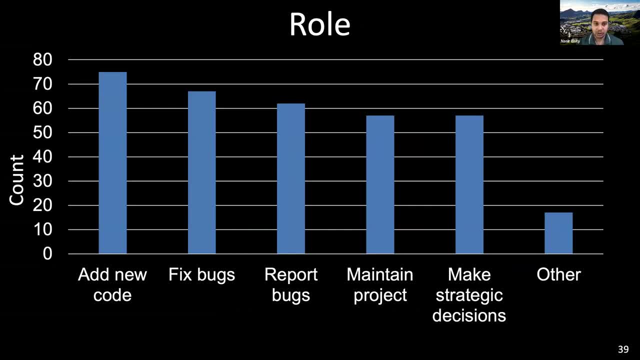 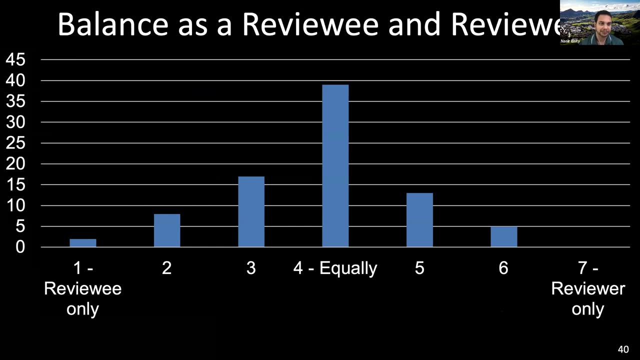 So this figure shows the role of the study participants, and then they assume different roles within their respective projects. It is similar to the first part of this talk that many participants play multiple roles, and this is usual in research software. And then we asked in a survey question that what is the balance between code they review and code they ask others to review? 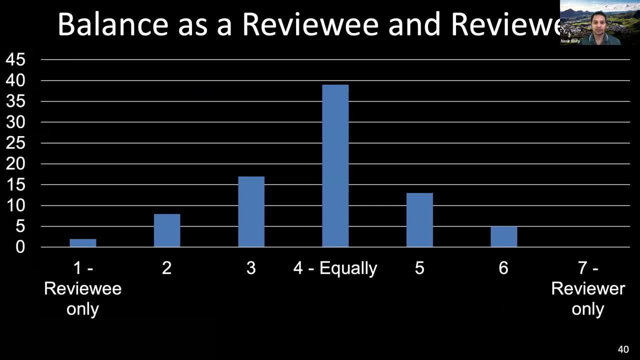 And the answers to these questions show, the respondents overwhelmingly participate both as code reviewer and reviewee, And only a small number of respondents act exclusively as either a reviewer or a reviewee. So an analysis of the raw data indicated that participants with more experience tend to review more, while those with less experience tend to write more with code. 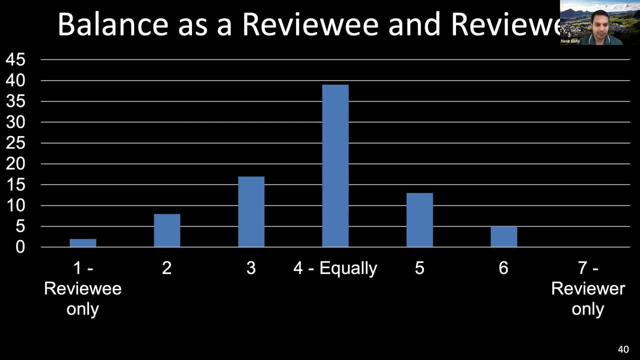 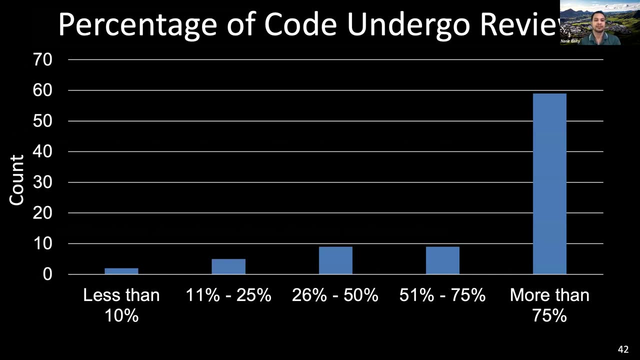 And therefore these study participants have appropriate expertise, both with the reviewing code and with receiving feedback from reviews, to provide valuable insight into the code review process. So how do research software developers perform code review? The responses to a survey question show that in the projects 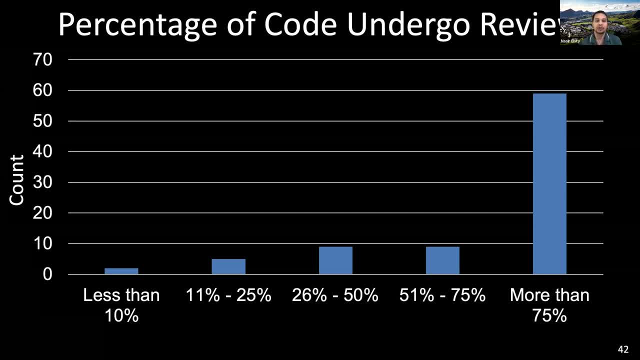 represented by the respondent, more than 75% of the code undergo peer review. A further analysis of the raw data suggests that in a larger open source of research software projects, only core developers perform code review, while in the smaller projects, almost all of the developers perform code review. 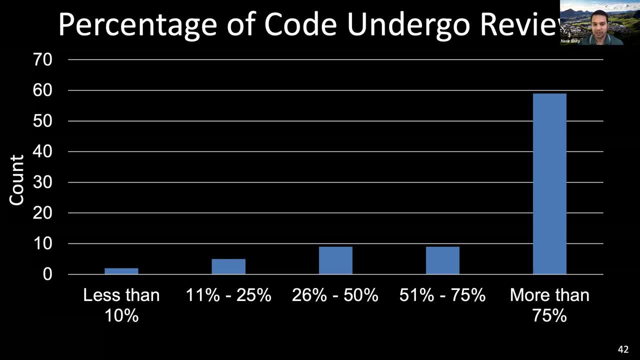 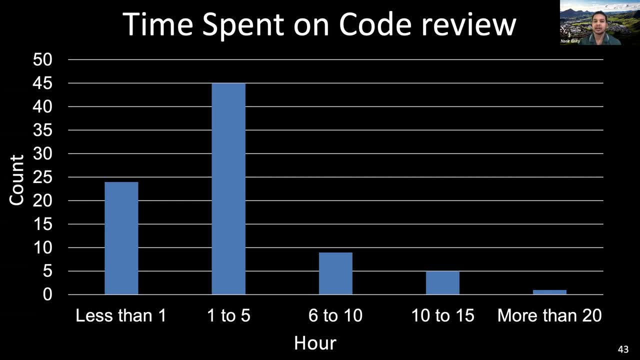 And this observation makes sense as participants in smaller projects have to take on more tasks. So this figure shows that most respondents spend one to five hours per week on code review, and an additional one third of the respondents spent less than one hour per week. Still fewer respondents spend more than five hours per week. 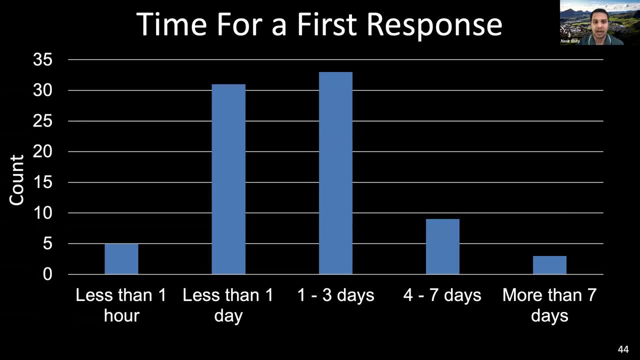 Time for the first response. This figure shows how long it takes a code author to get the first feedback on his or her code submission. Interestingly, 43% of the respondents said it takes less than a day for your first response, And the result is surprising. 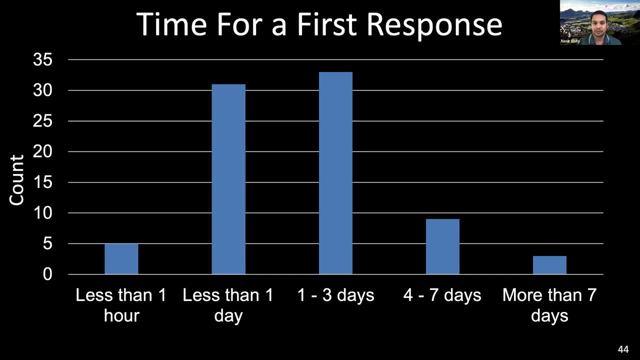 be. given that conducting code review is not the primary job of research software developers, nor do they receive incentives for performing code review, And approximately 40% of the respondents indicated the response time was one to three days. These results seem reasonable, given that research software developers 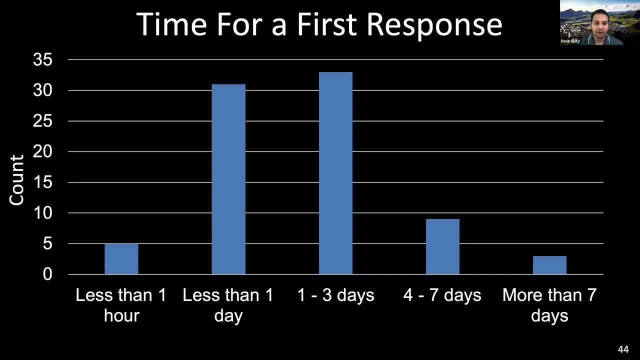 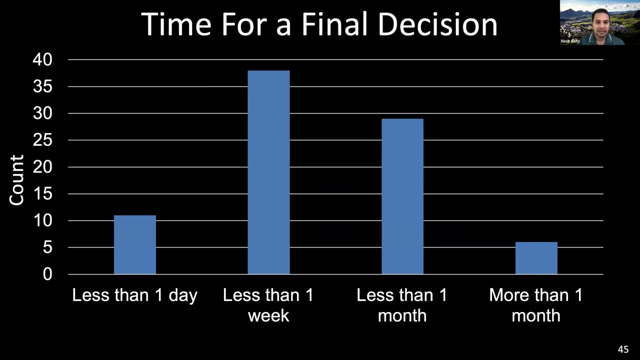 have other tasks related to their own work and may not prioritize reviewing others' code as quite as highly. The results in this figure provides an insight into the overall amount of time taken to reach a final decision on a code submission: Approximately 45% of respondents. 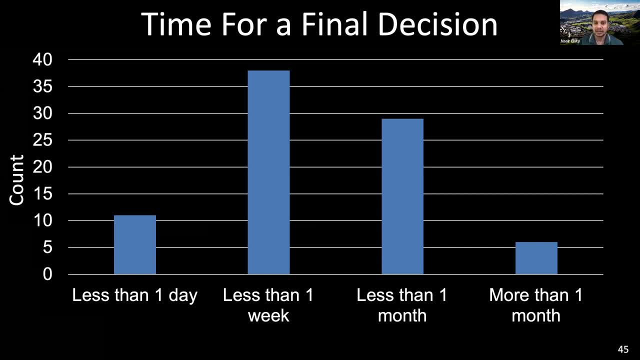 indicated the projects reached a final decision in less than a week, And for very small changes of bug fixes that time was even shorter, like less than a day. So overall, 93% of respondents indicated projects reached a decision in less than a month. 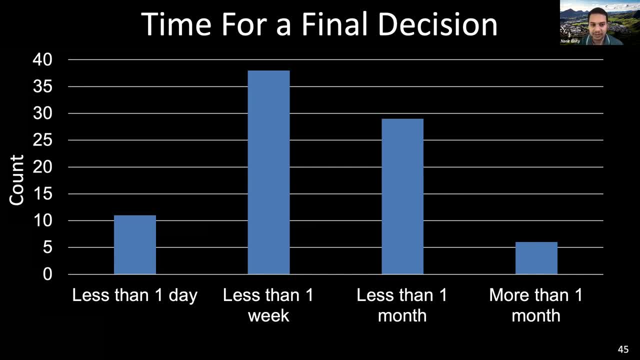 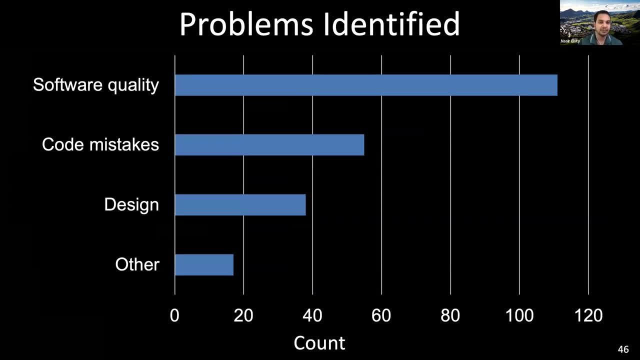 It actually depends on the size of the contributions, like small things could be accepted in a day or two, or a large thing could take weeks or even months. So code review help research software developers identify many problems in the code. So this figure shows three high level categories. 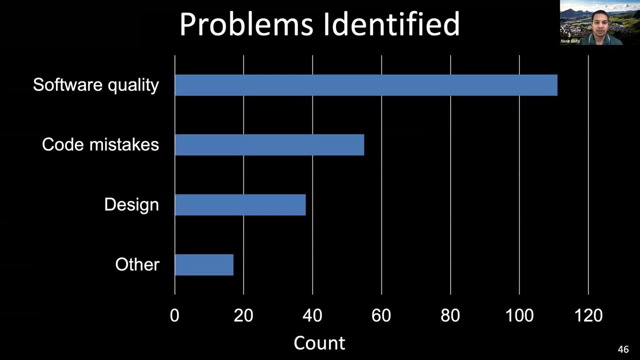 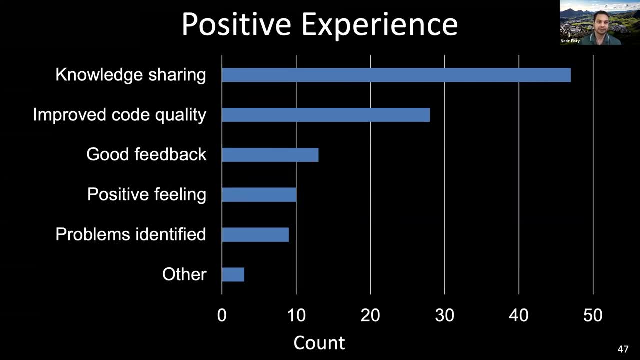 of problems reviewers identified. Most of the participants indicated problems related to the software quality and code mistakes. So we identified five categories of positive experiences research software developers have regarding code review. The most common positive response is knowledge sharing, So they find it to be a very cooperative process. 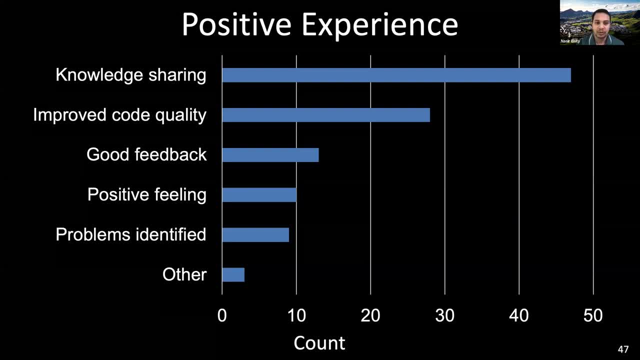 in which solutions are welcome and coders are looking for guidance. So they find it to be a very cooperative process in which solutions are welcome and coders are looking for guidance. So they find it to be a very cooperative process in which solutions are welcome and coders are looking for guidance. 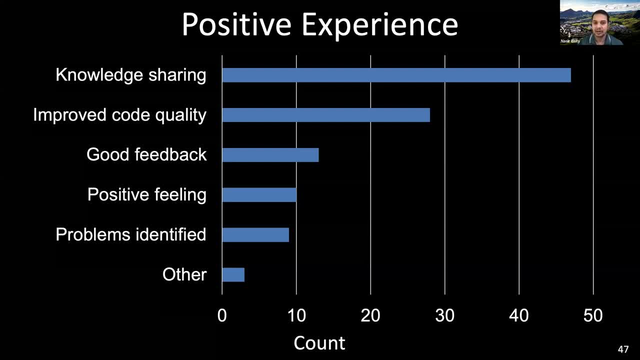 Also, in a big project, it is rare that anyone understand the whole picture and people rely on each other's experience with their part of the project. Respondents also mentioned improved code quality, good feedback, positive feeling and identified problems, So negative experience. 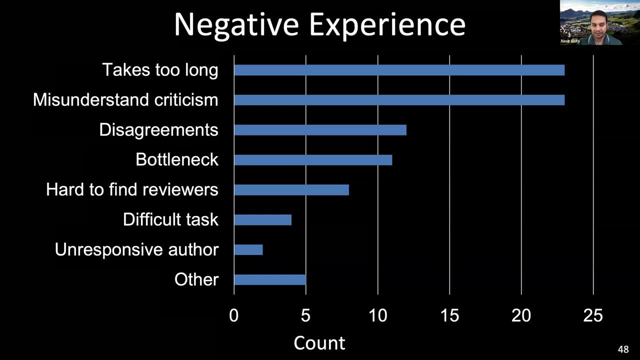 our analysis of the survey response is the: were the seven categories of negative experience? adaptive science or negative modelHOI or negative modeling, storage simples. you know 종ys cuk- surveillance, vision and forecasting. And then the conceptual focus to this was largely from information fiction. And then the conceptual focus to this was largely from the conceptual ourselves too. So there was a close 오케이 to them. weınd hasn't added any levar here. So to answer that question, just a open side question, for that You don't skills, You don't even understand it. 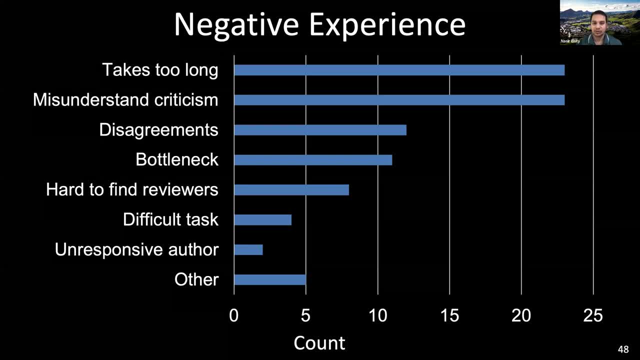 experiences. The top two negative experiences are that code review process takes too long and that the code authors misunderstand criticism The respondents mentioned. it can be very long and time consuming for very small changes, as the process must be followed for even a single character change. Now, when the author of the code misunderstand criticism, the reviewers are. 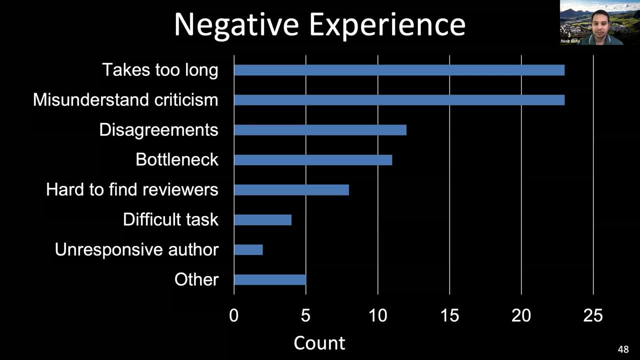 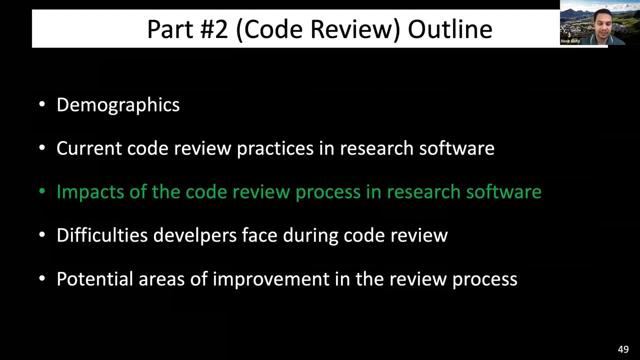 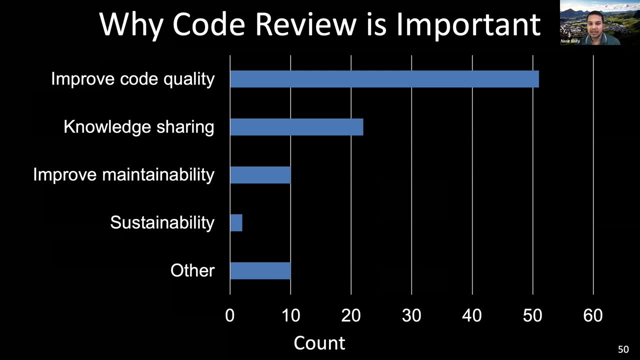 less willing to provide it or concerned with how it might affect the team dynamics. So what effect does code review have on research software? So in response to a survey question, 74 out of the 84 participants strongly agreed that code review is important for their project. Perhaps this result is not surprising, given that 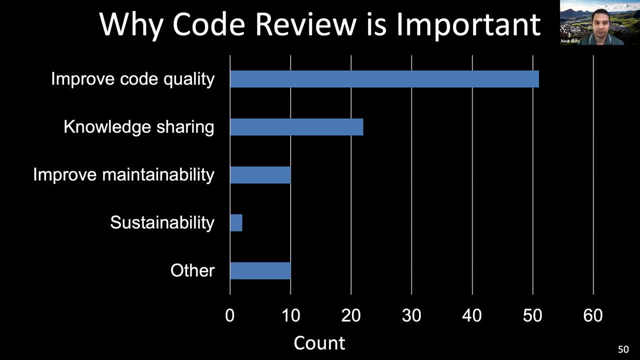 these people choose to participate in the project. This survey has a lot of information about code review practices, And then we asked: why do they think so? So this figure shows four primary reasons for the positive responses In terms of improving the code quality. participants said reviews. 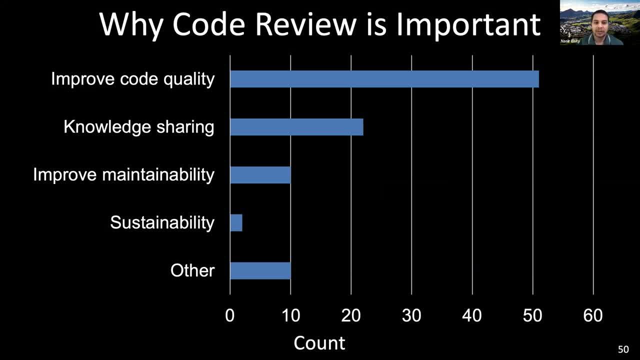 are a way to improve the code and learn. Without them, bugs would proliferate and code quality would decrease. It's a means of improving the code quality, the software or improve, or of improving the individuals who write it In terms of knowledge sharing, code review helps. 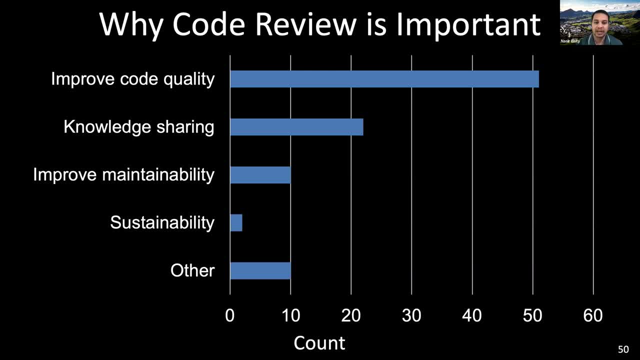 ensuring that at least two people have always looked at each piece of code. So it is spreading out expertise And, additionally, it is a forum for learning for each other, So people learn from each other. people learn from their PR developers and junior developers find it as a forum. 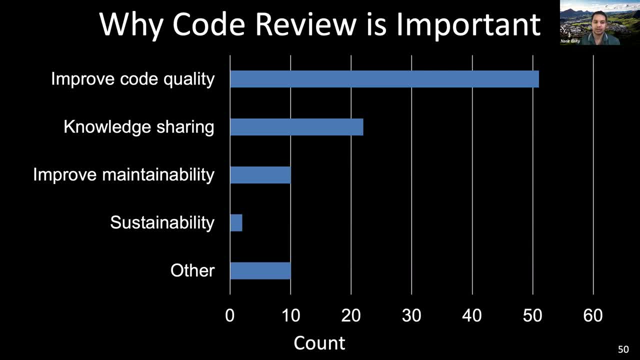 so that they can learn more about the projects, not only the code reviews. One of the few participants who did not think code review was important suggested that requiring code review as a compliance activity is a waste of time And, since that is their projects policy, he or she view code review as a. 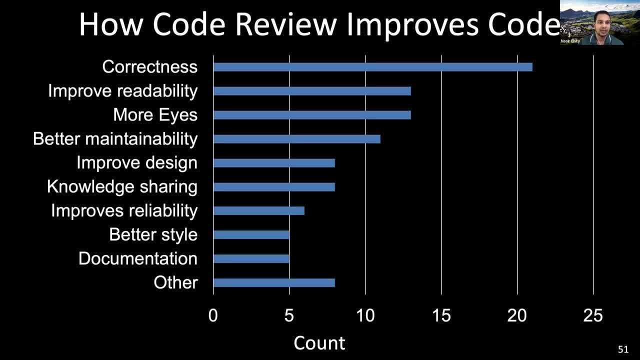 box to be checked: The how code review improves code. The most popular reason regarding improving the code was that code review helped with correctness. As one respondent said, if you have written the code yourself, it is hard to see the assumptions you have made. 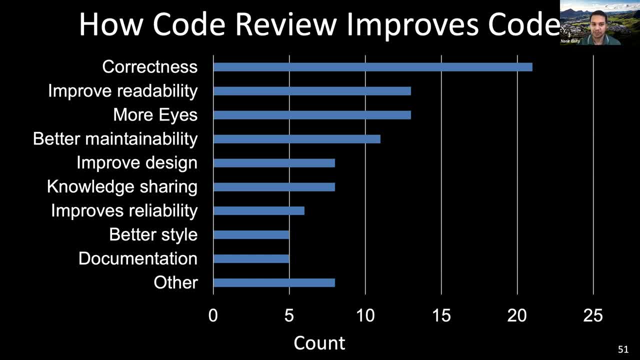 And others can spot this and ask you to clarify and spot your mistakes. Code review also improves code because it helps improve readability by making the code base more uniform And, in addition, having more eyes look at the code is beneficial because having a second pair of eyes often catches issues. the code author. 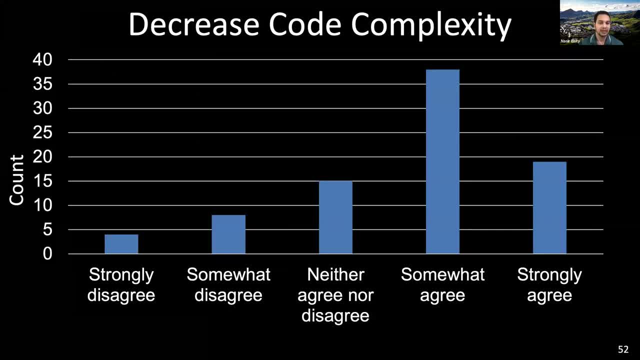 missed or did not consider. This figure shows that most participants agreed that code review helps decrease code complexity. For example, code review decreases complexity by solving problems using cleaner strategies, but may increase complexity in the near term by forcing it to handle corner cases that would not. 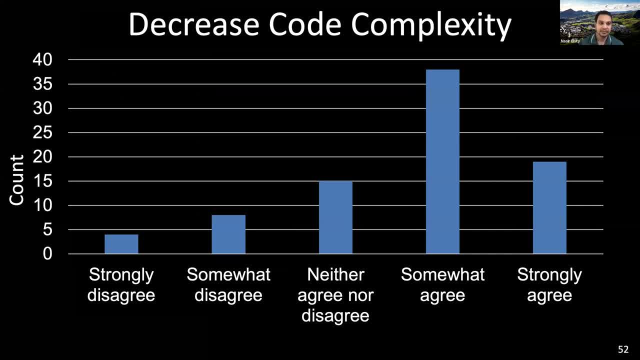 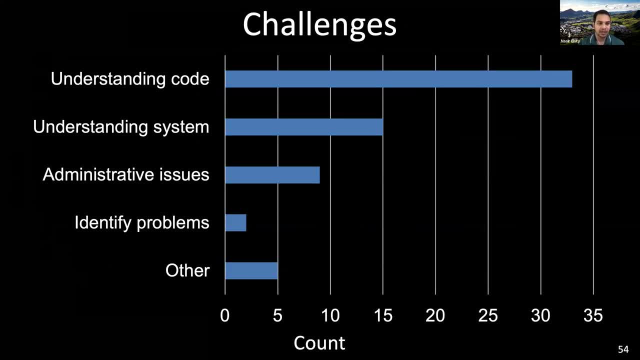 otherwise be discovered until later. So what are the difficulties developer face during code review? So we categorize the challenges of code review process into four high level categories. Overhelmingly, the biggest challenge is understanding code. For some respondents, understanding code is significantly harder than 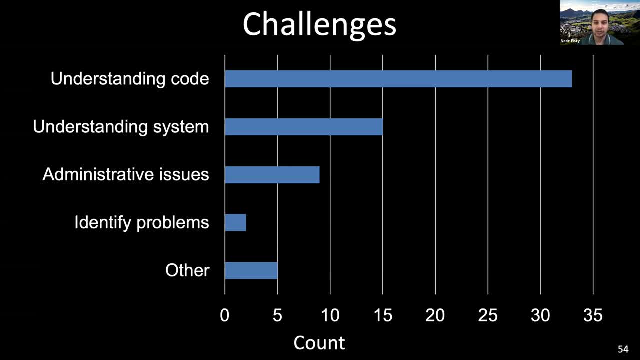 writing code And understanding someone else's code requires time because the reviewer has to work out exactly what added code is doing so that he can evaluate it. The other challenges are understanding the system, the administrative issues and identify the problems in the code. 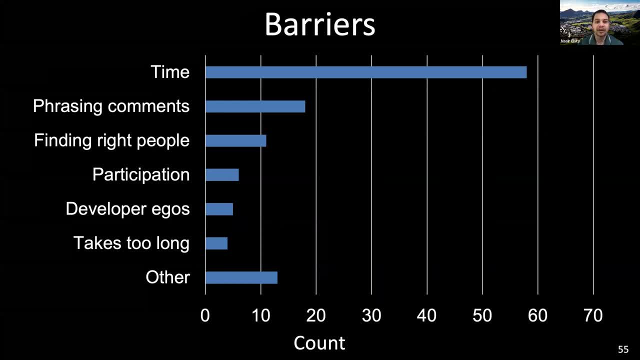 Then we found six types of barriers, And overwhelmingly the most common barrier is time, Because code review takes time away from the work anyone is supposed to be doing. The second most common barrier relates to the phrasing of comments, For example. often the reviewers don't dare to criticize code and 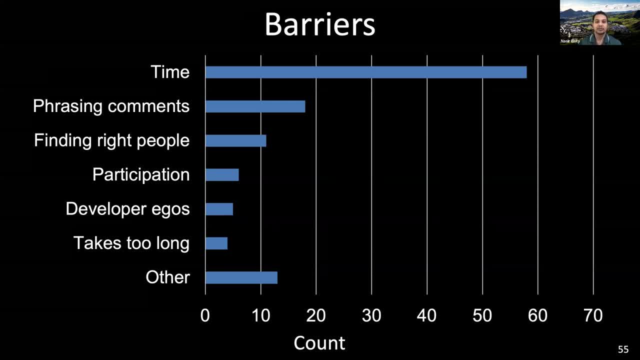 need lots of encouragement to do so, And reviewers are also concerned about how their comments are perceived, because there is no tone in written comments And another barrier is finding the right people, That is, people with both domain knowledge and the coding knowledge. So potential areas of improvement in the code review: 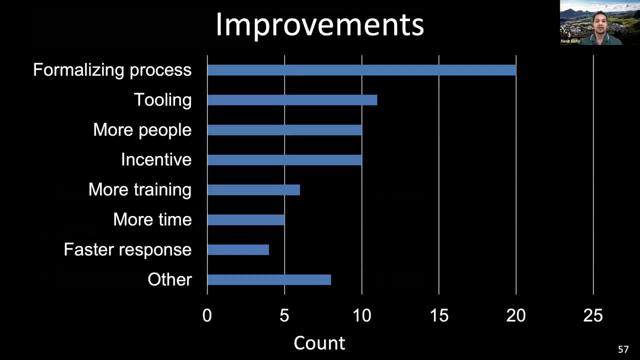 process. So our analysis found seven high level ways to improve the code review process. The most common answer is formalizing the process, likely due to the informal process followed by most research software developers, And automatic tooling could relieve some of the burden of the reviewers by making it easier. 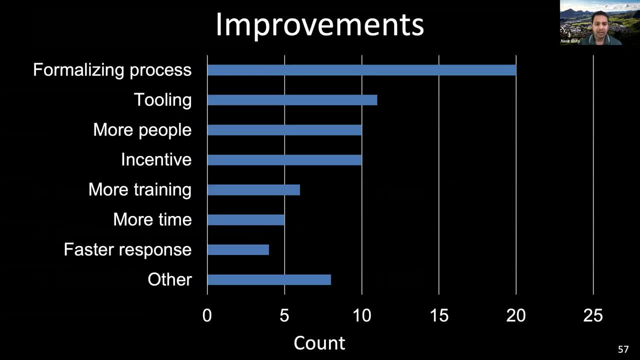 to switch between fork and branches in operation. Even though commercial and open source projects frequently use tools to support the code review process, many participants indicated the lack of tools, support for code review in research software And, finally, there is a need for more people. 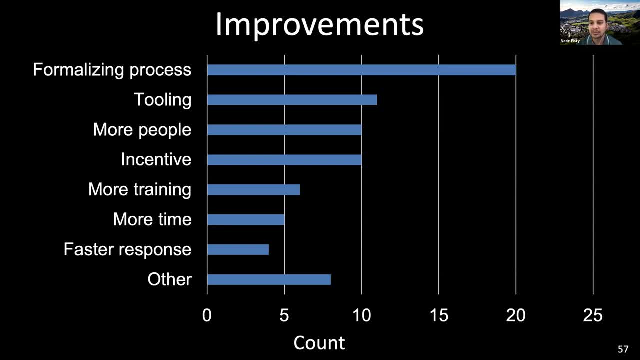 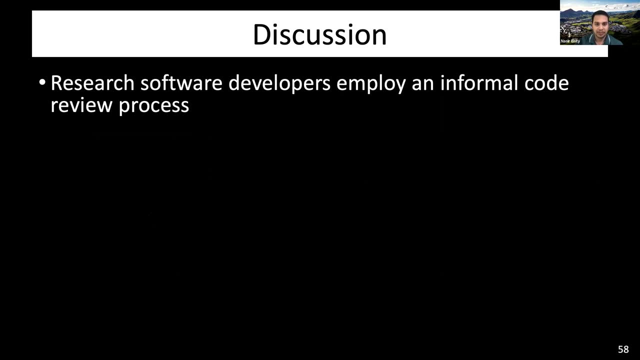 incentives and more training to improve the code review process in research software. Having said this, beside payments, some other kind of reward might help with that. To wrap up the second part, in general research software developers employ an informal code review process And code. 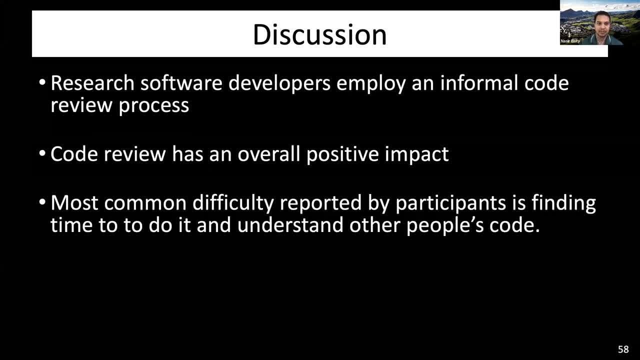 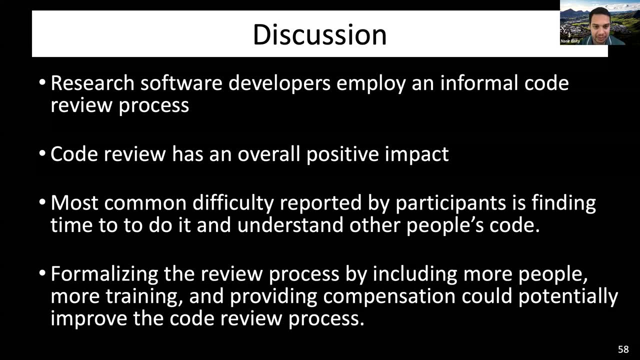 review has an overall positive impact and participants found code review to be very important in their project. The most common difficulty reported by the participants is finding time to do it and understand other people's code And so formalizing the review process by including more people, more training and. 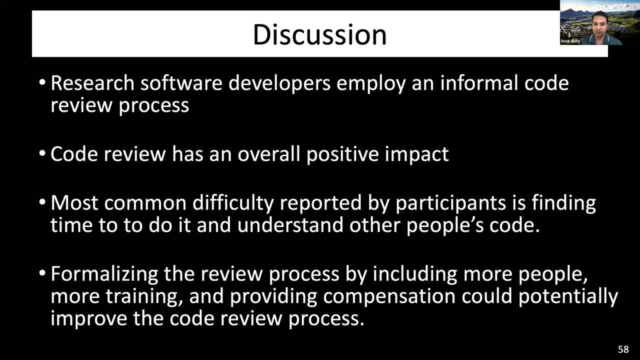 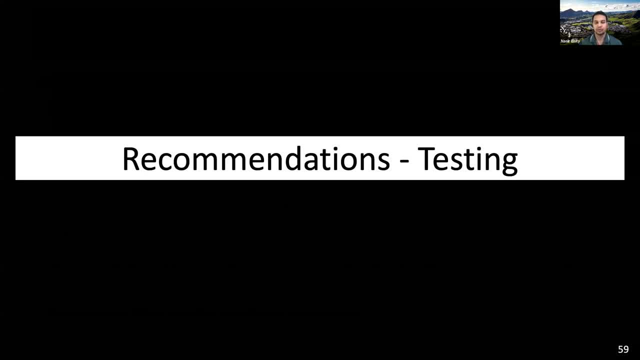 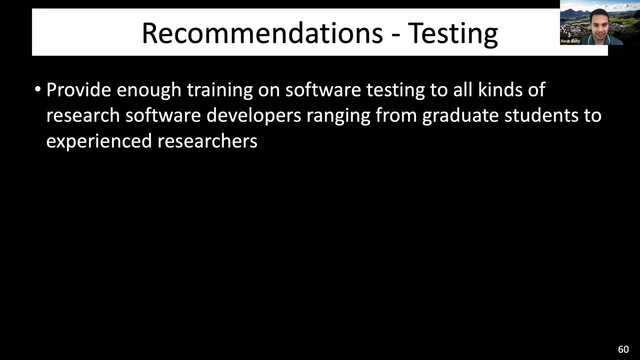 providing Compensation could potentially improve the code review process. So I'm going to provide some recommendations on both testing and code review. So, yeah, I may go ahead and do the recommendations first and then take on questions. So for testing, it's a provide enough training on software testing to. 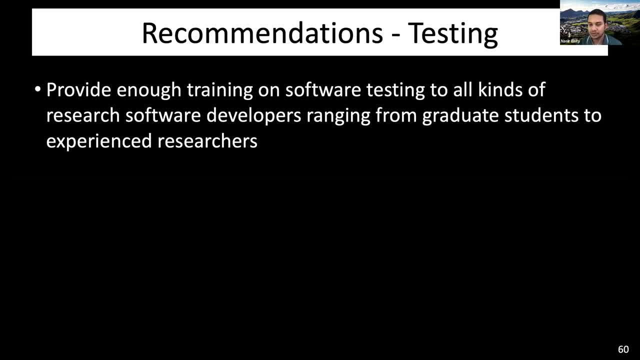 all kinds of research software developers, ranging from graduate students to experienced researchers. incorporate more tests that can solve the specific needs of the research software and provide infrastructure support, for example, a public service for training, including manager pricing structure, formation time and sophisticated testing dashboard. 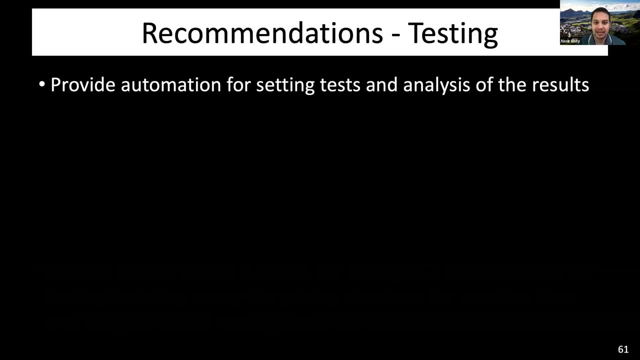 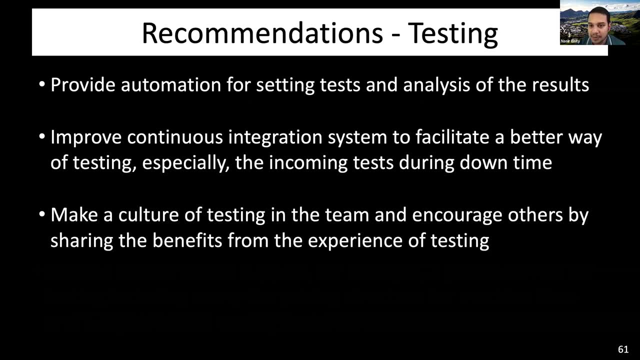 Provide automation for setting tests and analyze the result, And improve a continuous integration system to facilitate a better way of testing, especially the incoming test during downtime, and make a culture of testing in the team to an encourage other by sharing the benefits from the experience of testing and 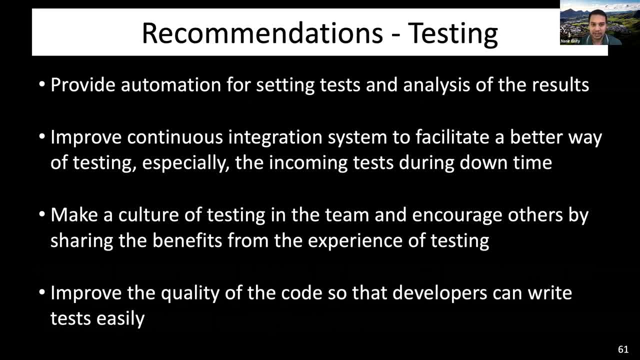 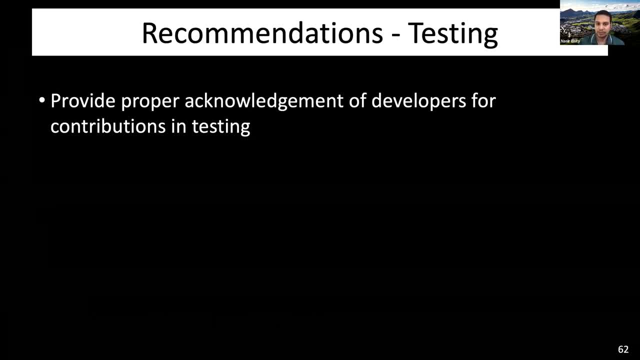 improve the code quality of the code quality so that developers can write tests easily As a. provide proper acknowledgement of developers for contributing on testing and make the testing process simpler so that it is easy to adopt in the project. and provide enough resources to developers so that they can utilize. 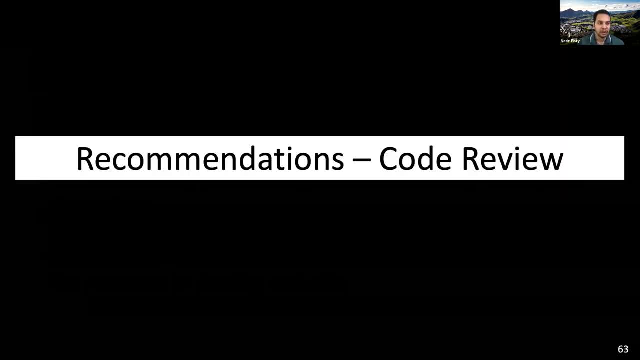 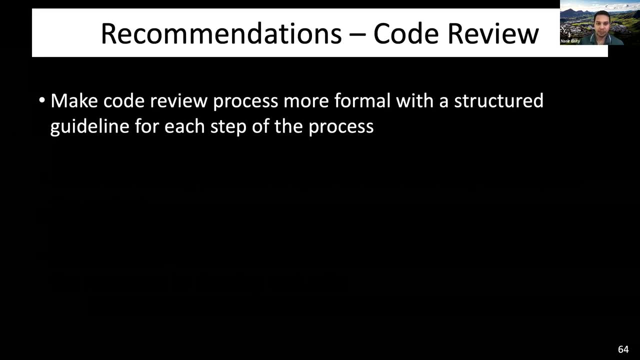 the resources to develop test suite. So here are some recommendations on peer code review. So make the code review process more formal with a structured guideline for each step of the process. Try to ensure at least one compliance review and one technical review. Include automatic 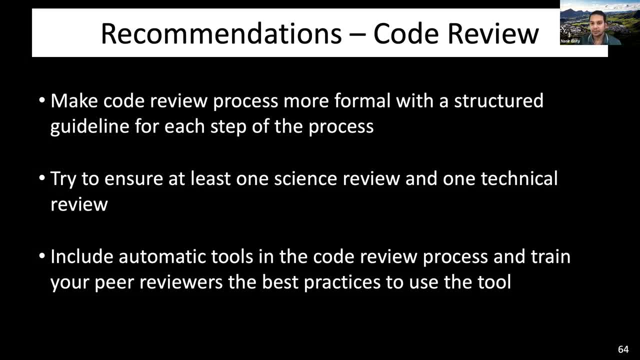 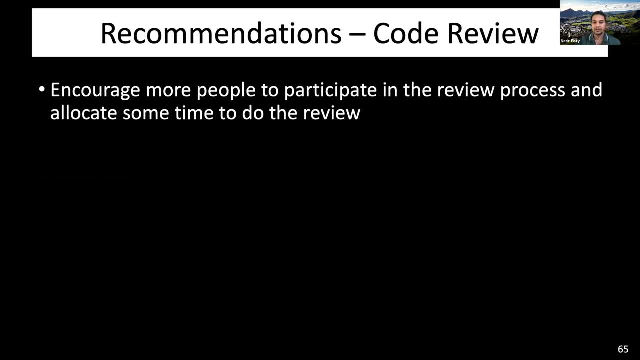 tools in the code review process and train your peer reviewers the best practices to use the tool. Encourage more people to participate in the review process and allocate some time to do the review. Provide incentives or rewards to reviewers to participate in code review. Allocate sufficient time in the 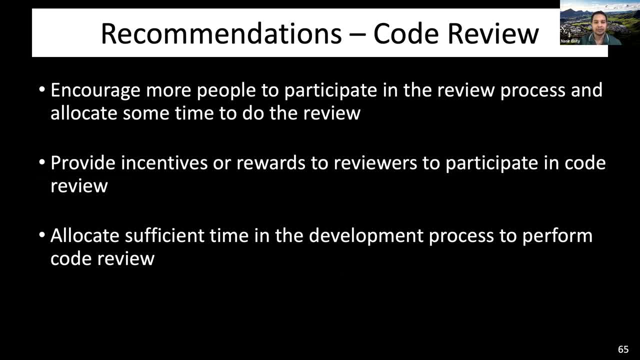 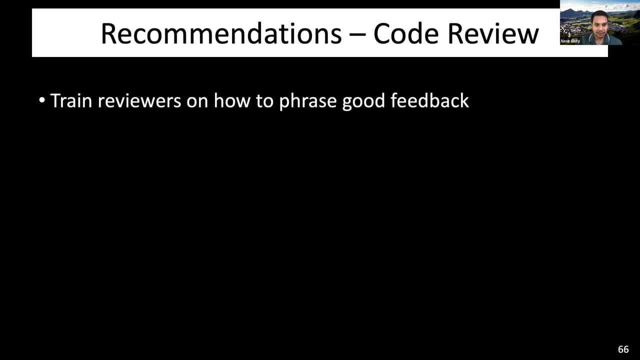 development process to perform code review And provide the feedback to any incoming review request, And train reviewers on how to phrase good feedback. and train developers to forget their egos and accept comments from the reviewers to improve their code. Make the overall code review process faster and provide. 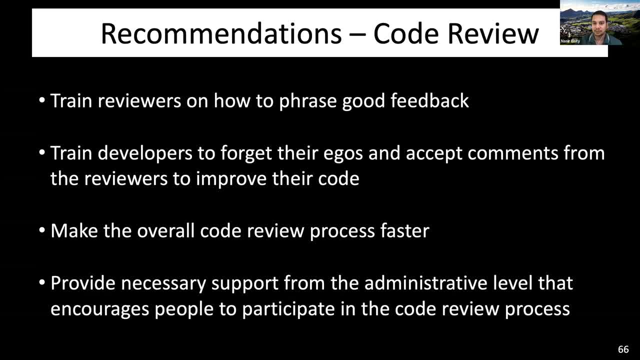 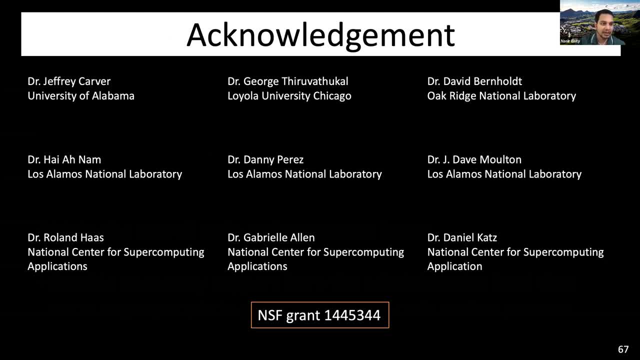 necessary support from the administrative level that encourages people to participate in the code review process. I would especially like to thank my PhD advisor, Dr Jeffrey Carver from University of Alabama, and all those good people from different national laboratories who helped me with these studies, And I acknowledge the support. 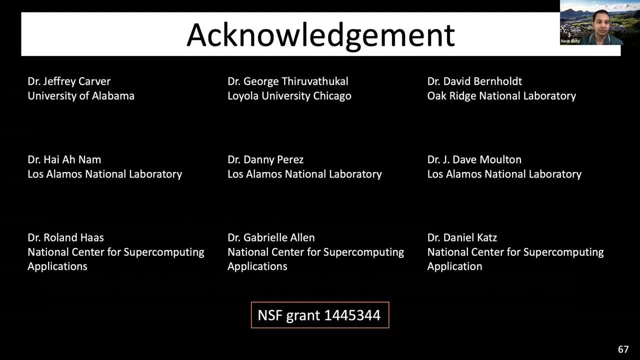 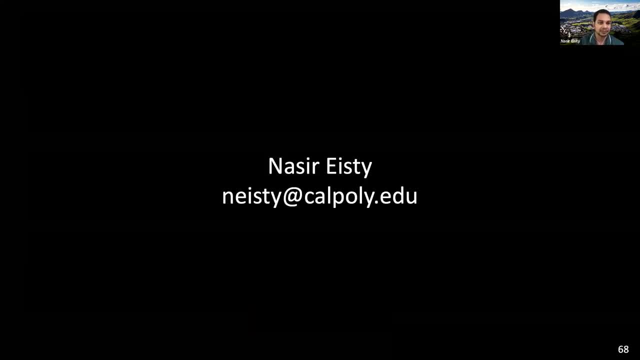 from the NSF grant and also I'm gratefully thankful to all of the survey respondents and interviewees for their valuable insight. So, yeah, this is my email address and I'll see you in the next video. Thank you very much. Now I can take on questions and go back to the Google Doc. Also, I would like to say at this point that if you are interested on software testing or anything on these, on your projects, feel free to send me an email. I'm looking for collaborators and also I have some follow up studies. I'm looking for teams and all that. So if you think this might be useful, please feel free to contact me. 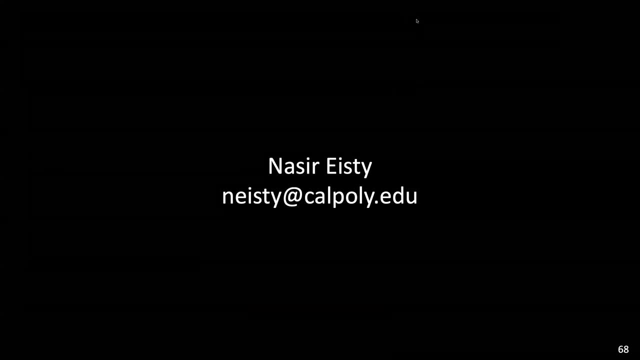 Yeah, thank you all. Thanks, Thanks, Nasser. So yeah, there's quite a few questions that are growing in the Doc. If your question doesn't get addressed within the hour, you know right now that we can, that all the questions will get addressed, And so you know, come back to the Doc at a later time as well. 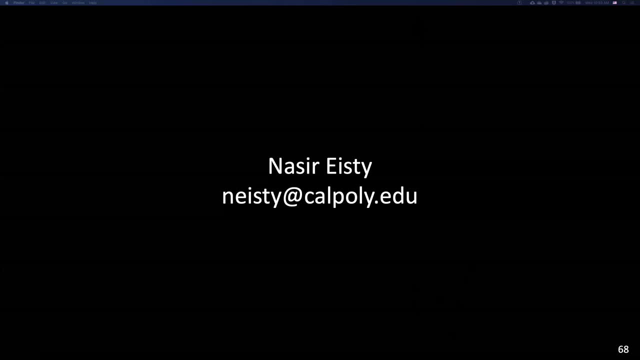 I just want to say you know, thanks. I can tell you are a new father, a new faculty and a new Californian. I appreciate the presentation amidst all the craziness that is going on in your life. So thank you very much. 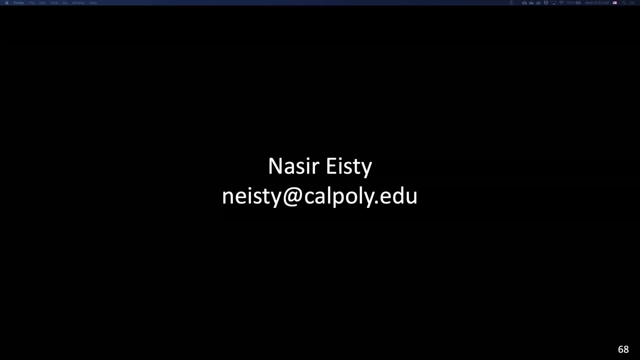 All right, So let's go back to the questions then. David, can you help with moderating some of the questions, Maybe some of the ones we can address at this time? Sure, I'm looking at the question document. There's a lot of people who are really interested in finding links to resources and I think the best way to address those might be by typing into this document or providing further links. 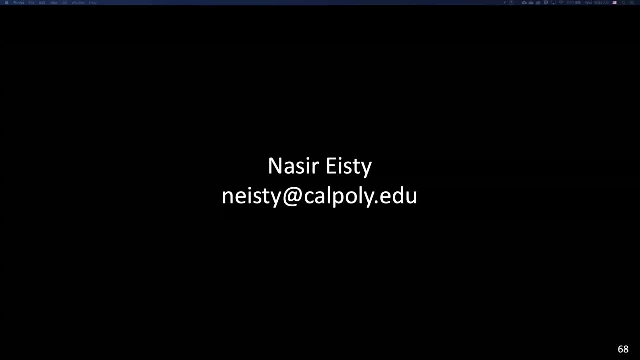 So I'm going to focus here on questions that are about the research, surveys and recommendations specifically. Yeah, I can see a question for 50 definitions of the survey, So I still have the link of the survey, Let me. let me write it down here. So that was circulate testing. 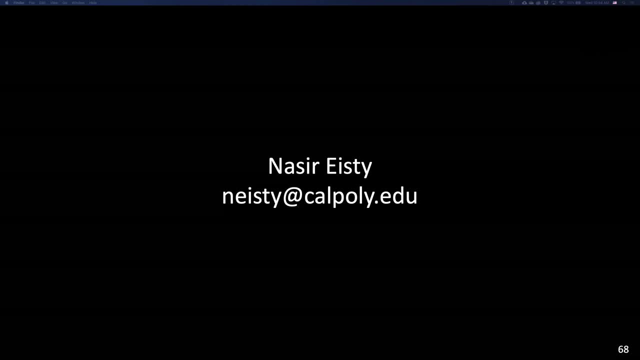 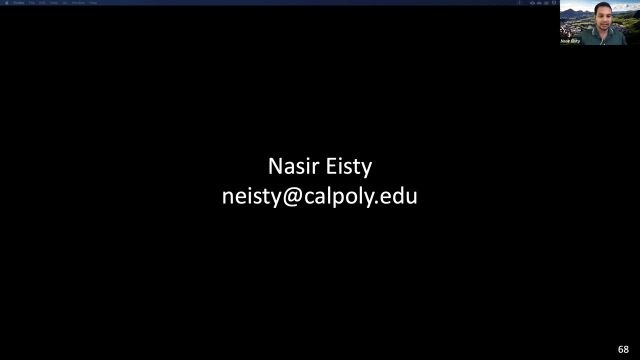 DSSW testing survey. Yeah, I got it, So the surveys is still live. for the definitions of research questions, Take this: Yeah, Yes, So I posted a link So you can find the survey over there. The definitions are still over there, I think It's live. 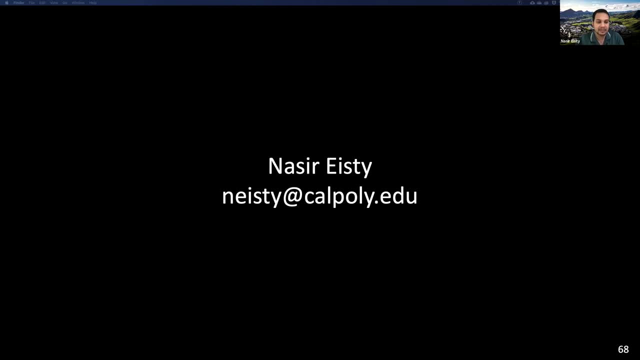 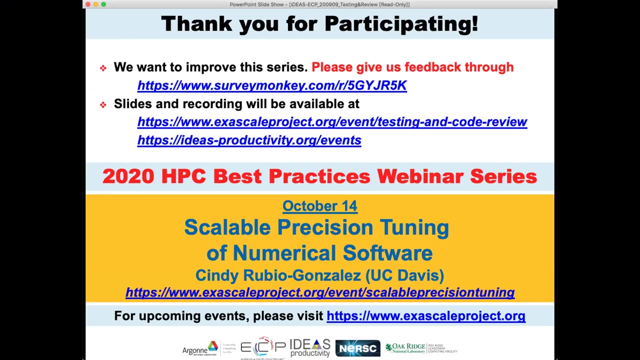 Oh, I see. Is there a The survey link? Yeah, this is the survey link that we sent last year. Is that one that we just posted to the chat? Also, Survey Monkey 5GY. Check on that So I can stop sharing the screen, right, Or do I need to keep my screen shared? 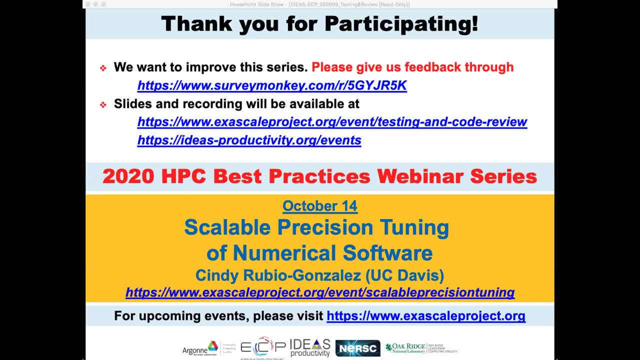 So I kicked you off and I have listed the. This is the closing slide for Now I can see the chat. Yeah, Okay, Yeah, This way, Yeah, because. so for anyone who needs to drop off, I just want to remind folks that the next series is October 14 on scalable precision tuning of numerical software. 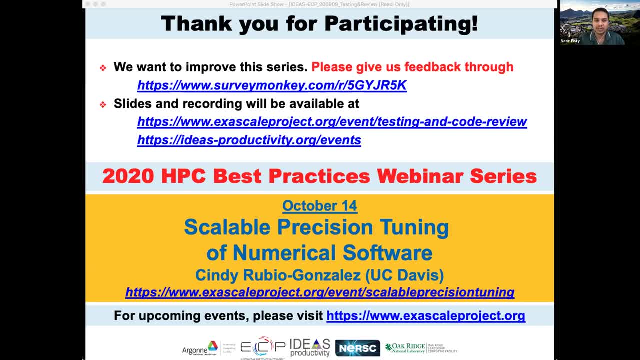 The survey link I posted on the question and answering document is the testing survey where Someone asked the definitions. So if he goes to that link he can find it. Find all the definitions. Okay, I see it now It's: It's BSSWio events. 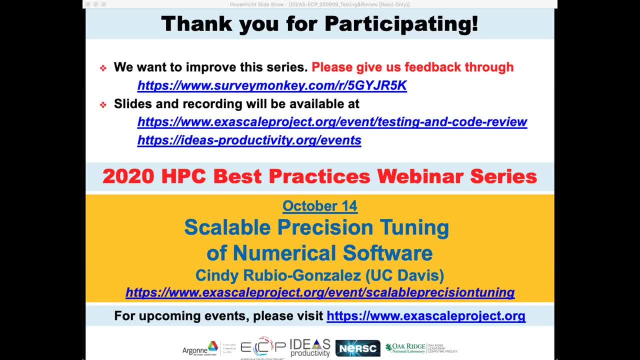 I events? Yeah, And for future reference, If we go to this BSSWio events page will be fine surveys that you put out, or how how can we get connected to your service? Yeah, So in on the event space You can find all the service, Yeah. 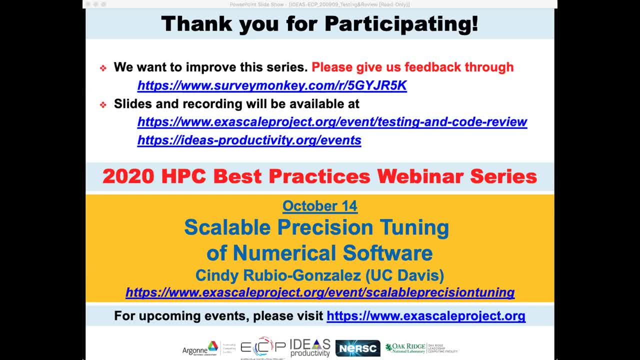 Right Now, There was one question on what did commercial it methods refer to? Is that She liked him into three? Yeah, I think it refers to the unit testing, integration testing system, testing and acceptance testing and all this. Yeah, These are the methods. Yeah, And so these methods were actually generated from the testing practices in the commercial IT software. so 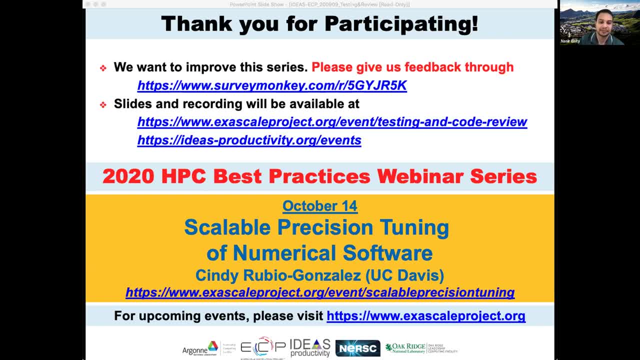 Nowadays people call it like commercial IT software methods. Okay, Was there any study? is Respondent bias? It seems likely that people who do testing would be more likely to respond, and the results for research software in the wild might be worse than presented here. 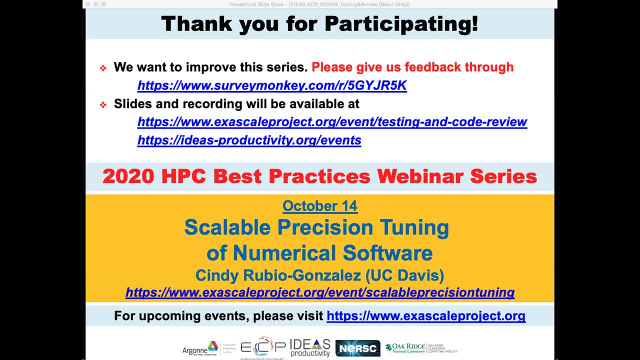 People might have been biased to be more favorable towards testing because they answered a question on testing. Yeah, that's true. That's true. So that's the limitation of the survey. So if someone agrees to take the survey, So that means he has some sort of experience or some sort of interest on testing. 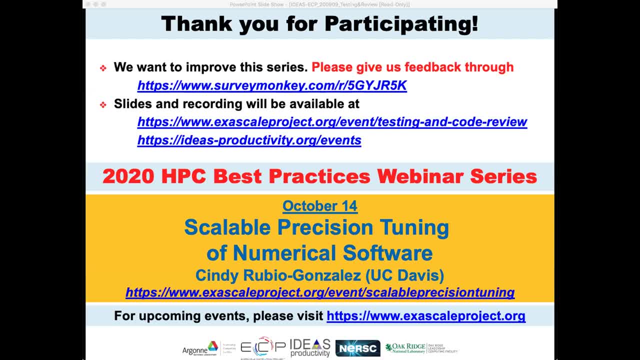 So this might be a little bit Biased, but yeah, that's true, But that's the best we can approach. for Okay, but was there a question specifically that you might look at as Familiar? familiarity with testing practices, So which? So where is in the doc you are asking the question is in the second page or first page. 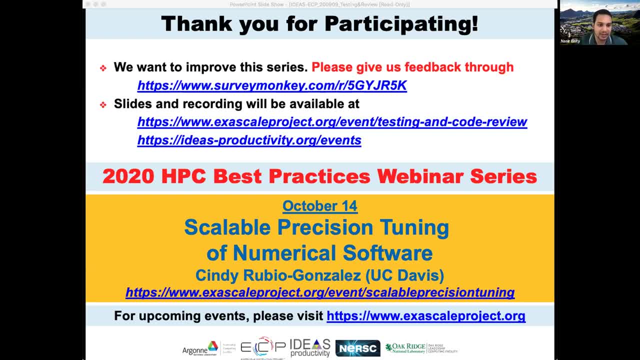 I am highlighting it here in the second. Okay, so was there any study of survey respondents bias, So the So these are all published Or in the process of publishing actually. So these are. both of these studies are journal paper and that will be coming out late this year because I'm working on the review and the revision of this. so 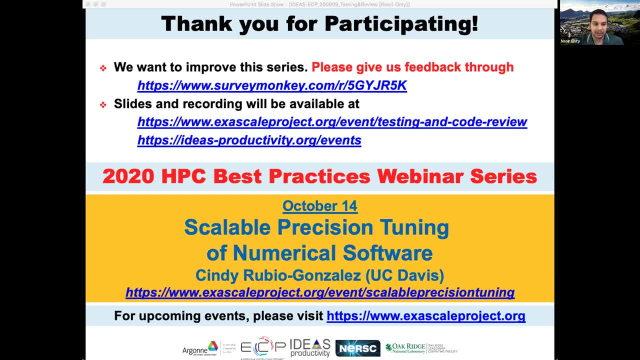 You will get it published and maybe we can send out and mailing list email that the paper is out. So there are more results and there are more explanation. So because of the talk, I had to make a choice: to pick some and don't pick some. 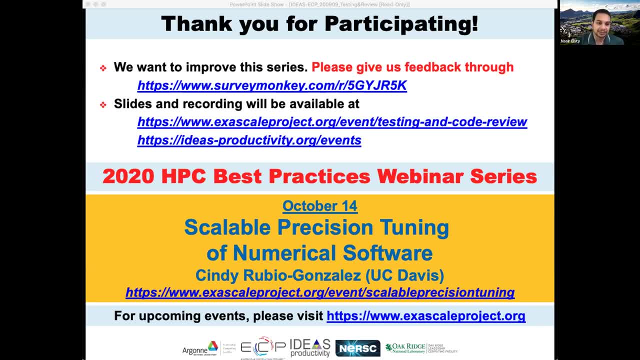 Okay, Okay, And so in the limitation You can see the study survey respondents bias and also it seems like the people do not be more likely to respond Yeah, and I agreed on that people who do testing would be more likely to respond. Yeah, that might have happened, but we did not track on respondents and we don't collect personal data. 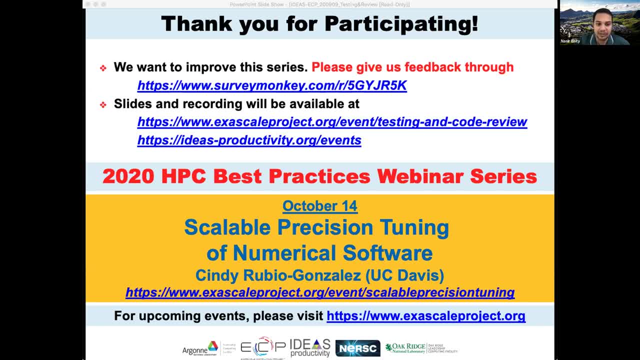 So we can say that: But yeah, that's the trade. That's the trade to the study That might might be biased and and this is how empirical studies actually work, because anyone, anyone wants to do some, Anyone wants to take this survey, or anyone's agreed to participate in the interview or any sort of data collection So he or she might have some interest. Otherwise, he wants to spend time on that. 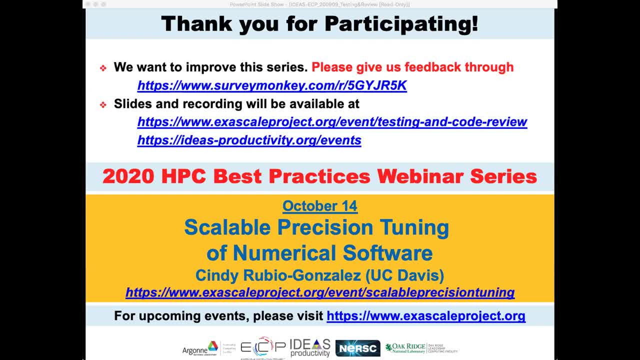 And how does team size affect code review practices? or have you looked at the correlation? Yeah, so The team says really effect. So when there is a lot, There is a big team, There are more people, so people can put aside some of their task and and do the reviews. but I 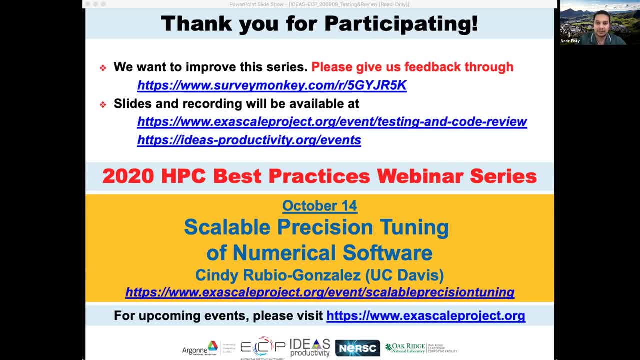 I have seen some teams that are fairly small and they have. they have more roles to take on and they do more work, so they don't really get much time and and much resources, and it's smaller teams is that it gets less resources. So, yeah, a lot of the teams that tend to do more. 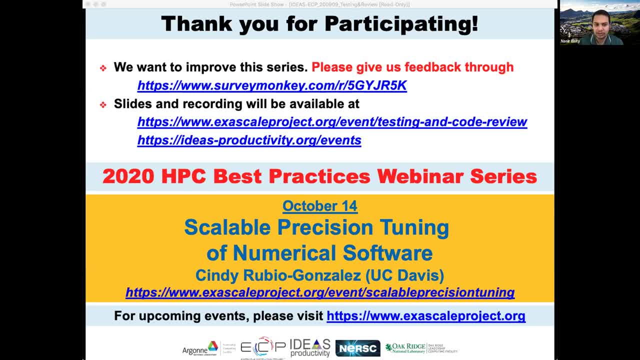 So I work on a team that has more than 100 developers all around the world and they really do code review more formally and and core review- the must for them to have the past March to the repository. but for a small teams and sometimes the people and the folks just work directly sitting on a room and they're just informally. 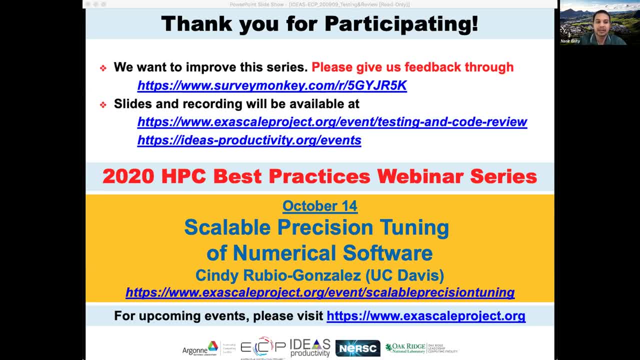 Show each other's code and do the reviews. So I think larger teams teams have much more formal code review process. Okay, it's two o'clock and we're actually out of time, but thank you for answering the questions we were able to get to. 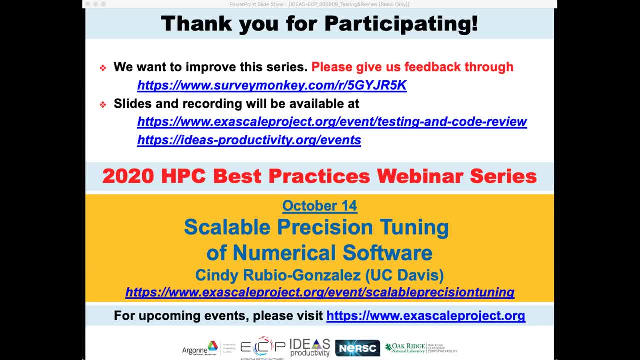 The rest of them, I think we'll be typing in answers and providing links to resources. Also, in a few weeks time, this recorded session will be posted. Okay, so I wanna add that I will go over all these questions again and I will type in: